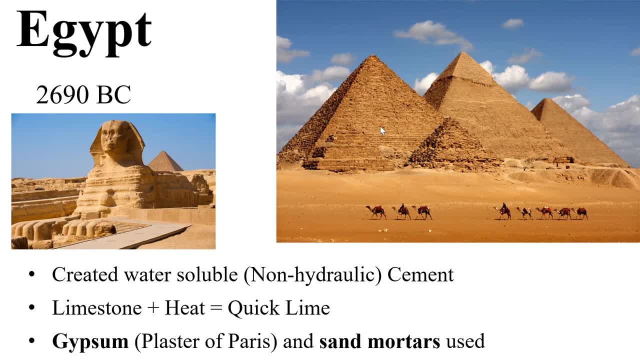 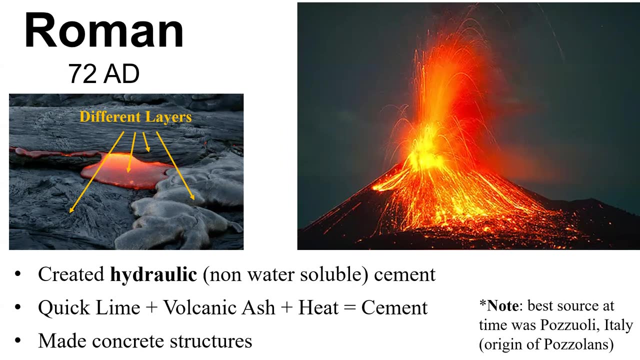 But the pyramids they built all sorts. There's a bunch of stuff over in Egypt, you know, with quicklime, the same non-hydraulic cement that we just talked about. The Romans actually got a little more creative. They figured out the issue with the water and they were actually able to make a non-soluble, so non-hydraulic, so hydraulic- sorry, a hydraulic cement. 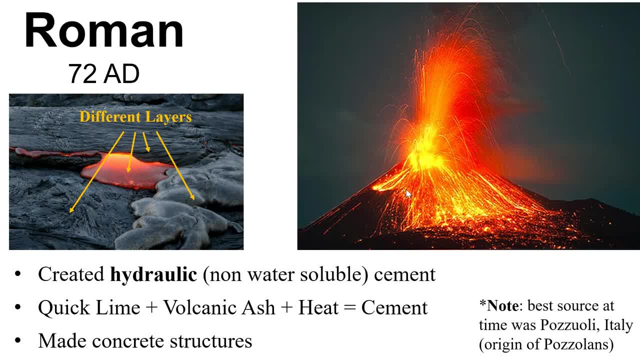 And there it was kind of cool how they did it, where they actually realized when they looked at the volcanoes and these different lava layers came out. some of them would be what you think of with like lightweight aggregate, some of the layers. 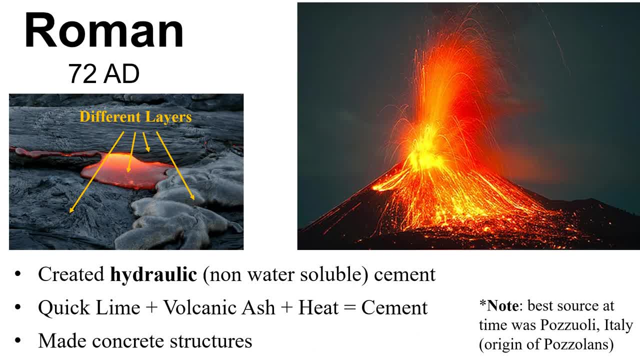 You know, you go out and you grill a steak with your grill and maybe you have those little bitty lava rocks that you're using to grill with. Actually, they look very similar, Very, very similar to stuff like lightweight aggregate. Some layers were like that. 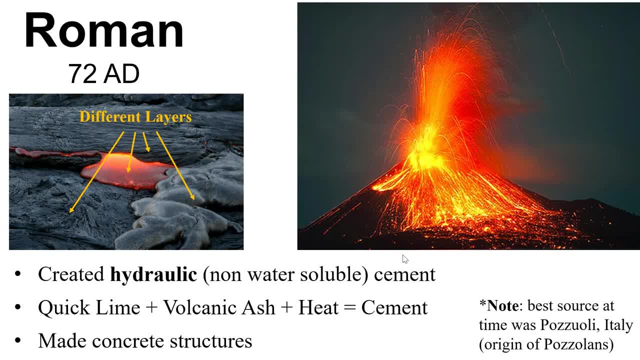 Some were more of like a fly ash that you'd think of here, And there's some that may actually have been a hydraulic-based, more of like hydraulic-based cement, But what the Romans found out was, if you took some of this quicklime, so the cement that's not, you know, that's soluble in water. 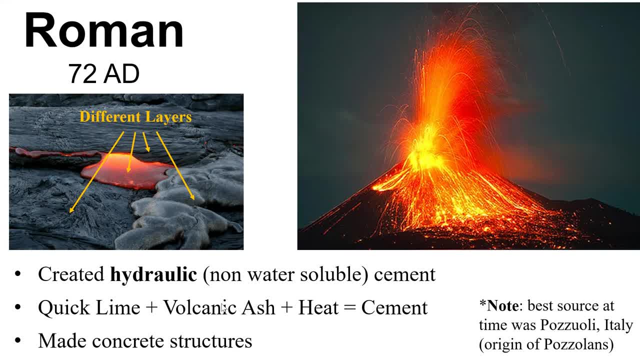 and you took some of this volcanic ash And then you heated everything up. you could actually make some cement with it, a hydraulic cement that didn't have all these water issues. So it was really cool, And one of the best places for volcanic ash was in Pozzola, Italy. 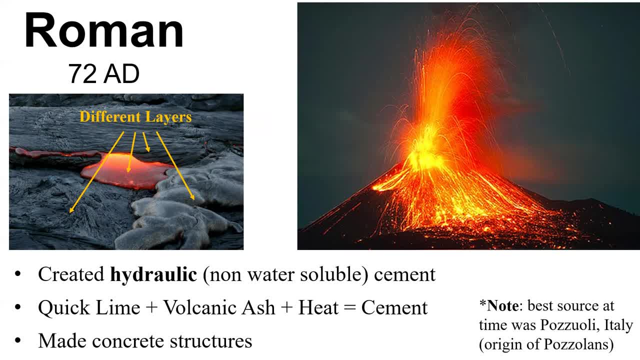 That's actually where the origin of pozzolans came from. So in this class you might hear secondary cementitious material. You hear the word cement. You hear the word fly ash a lot And you know people associate the word pozzolan with maybe like a class F: fly ash is a pozzolan. 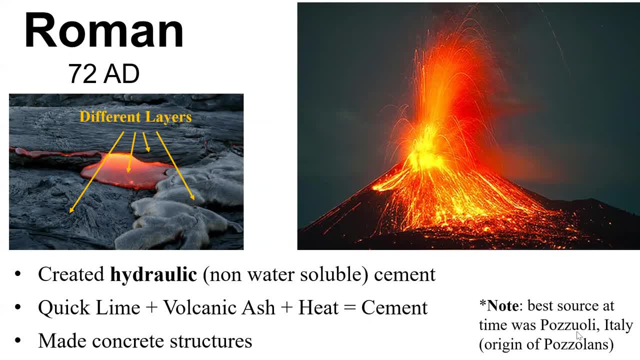 And what that is is in essence, it's very similar to what you think of it with a cement, how it looks anyways, But chemically it reacts differently. So it reacts at a much lower rate And you're able to replace a certain amount of Portland cement with a, say, a fly ash. 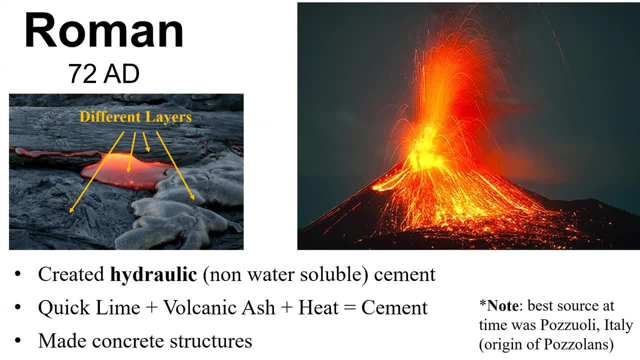 These are commonly at 10 to 30% for fly ash And they actually can enhance the performance of your concrete. So, just kind of a side note, We'll talk a little bit more about secondary cementitious materials and fly ash and pozzolan. 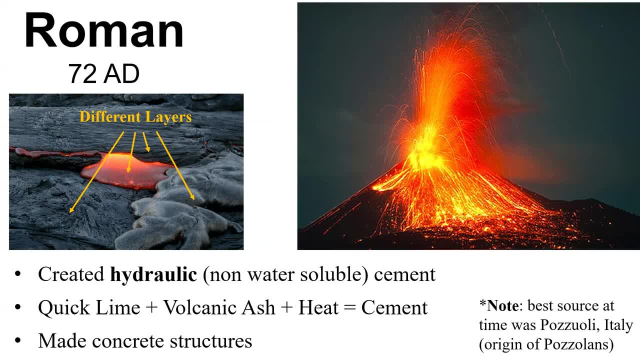 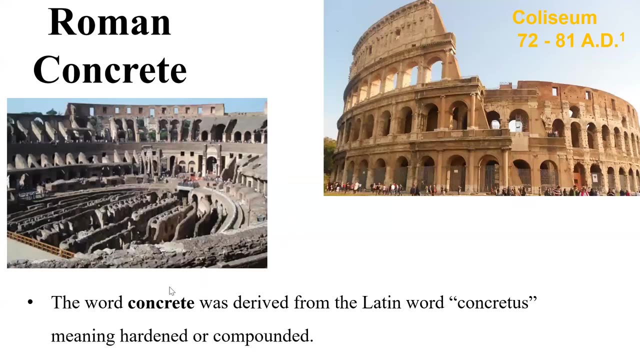 But I just kind of wanted to throw that out there, just in case you were kind of familiar already with what pozzolans were. So the Romans, they took this cement, this hydraulic cement, and they made all sorts of different concrete structures all over the world. 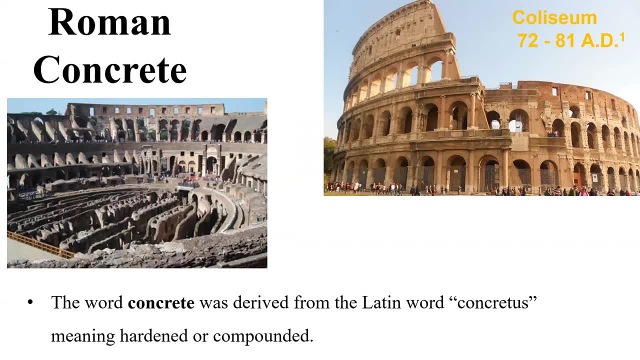 And the word concrete is actually derived from the Latin root word concretis, meaning compounded or hardened, put together, And so they built a lot of different structures. Some are actually still standing today. There's a lot that they built that didn't do very good, and they're no longer here. 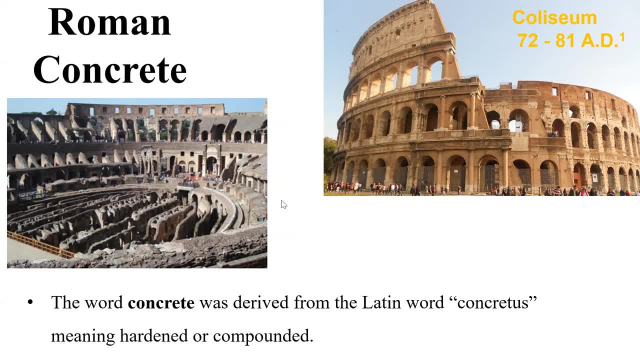 But the ones that were really good, the ones that had the best materials, the best craftsmanship, they're still around. You know the best design too. So you know all three of those craftsmanship design and the actual, you know, using the right materials. 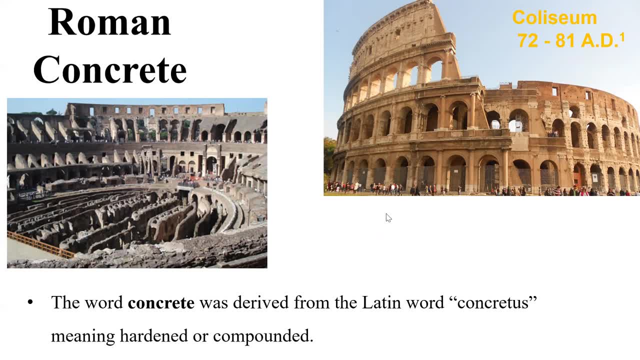 You know, actually it's a lot of different things, But what you find with most engineering, that's actually what happens. So if you want to have the best structures, you better have good engineering designs, You better select and use the right materials. 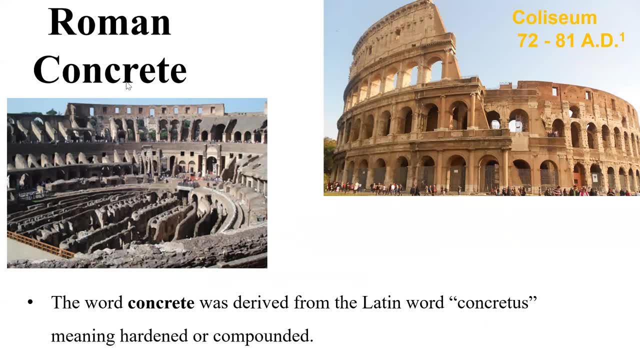 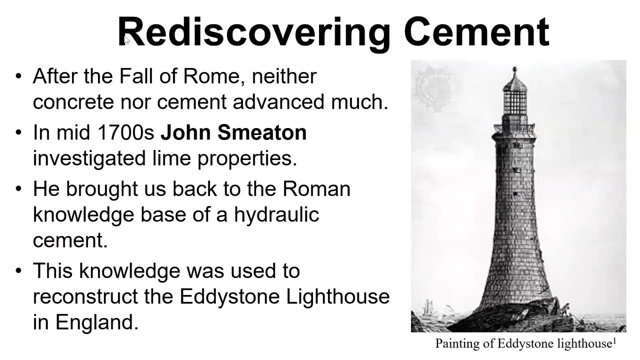 And when you're building a structure, you need to have a minimum, you know, quality of work And you know and these structures will last a long time. So, unfortunately, the Romans figured out all sorts of different things, But they actually, you know, they had the fall of the Roman Empire. 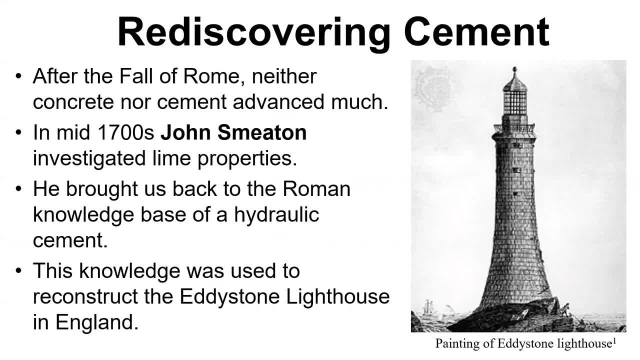 And they actually lost a lot of really good information, a lot of good resources, And so you know, then you had the Dark Ages that kind of came in And nothing really happened. with cement, with concrete, Neither one of them really advanced much. 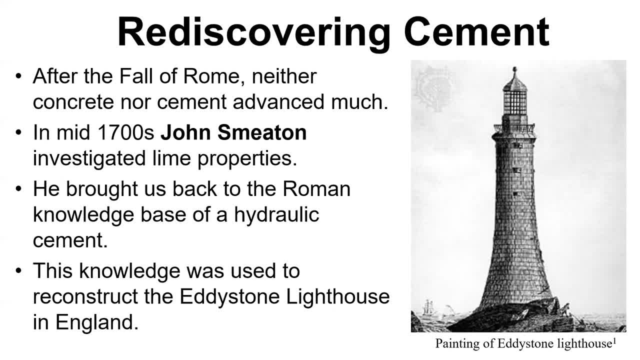 And it wasn't until the 1700s, with John Smedon, where things really started progressing. You see, in England, you know it's on an island And the shipping from all over the world was a big deal back then. 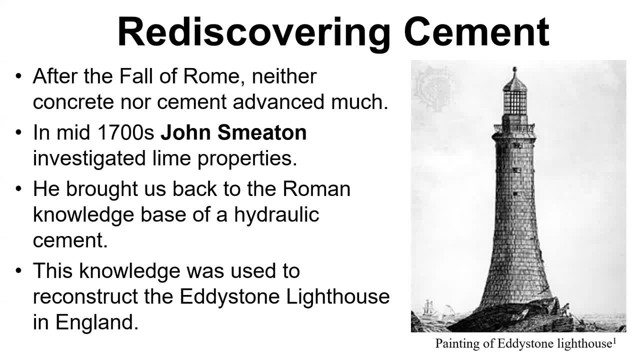 And they really needed to figure out how not to ruin their boats, because you get too close to the shoreline And you're going to wreck your boat, And so you put lighthouses to kind of say, hey, you're pretty close to the shoreline. 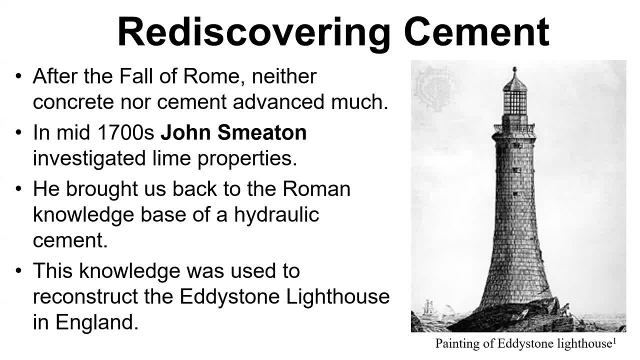 You need to be cautious. It's right here, But these lighthouses didn't last very long in these very corrosive sea waters. So what John Smedon did was he started investigating line properties, started really looking at what exactly would be the best building material to use on these light towers. 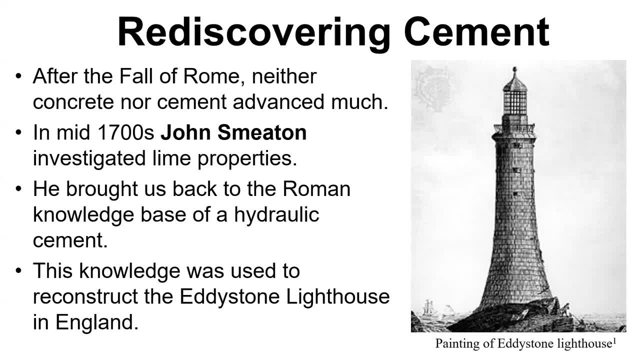 You know, wood didn't really work, Steel wasn't really work, Metal, I should say, didn't really work too well. But you know there seemed to be something with the lime And really he started doing so much research and looking at stuff that he actually brought us back from. you know pretty much where the Romans were with his basic knowledge of hydraulic cement. 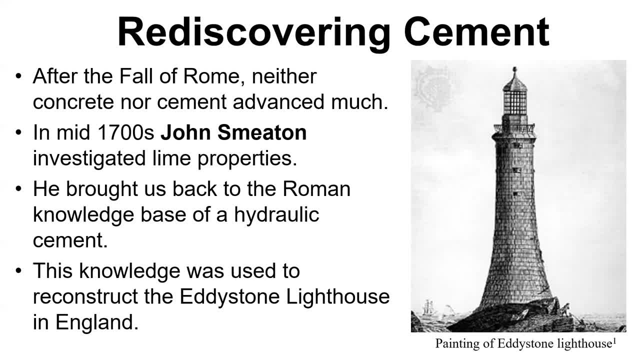 And it was kind of cool. Yeah, So John Smedon did a lot of research about how he brought us there And you know, in essence his big, you know, name to fame was he actually developed this Eddystone lighthouse, which lasted a lot longer than all these other lighthouses. 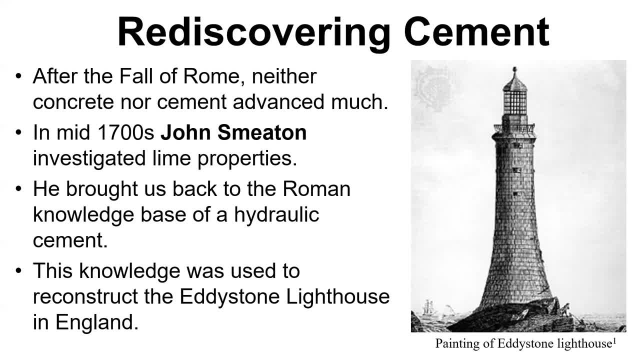 It was built really well And these ships wouldn't go and crash as much and lose a lot of their cargo, So it saved people a lot of money. Also, I should note that John Smedon is actually the first. He's what's considered the father of civil engineering. 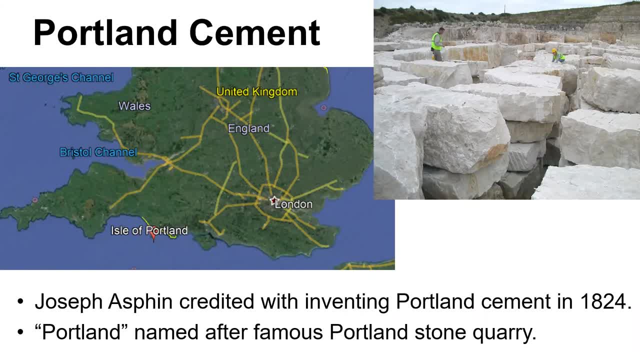 And many different discoveries occurred right after John Smedon. So Joseph Aspen, just you know, in the 1800s he actually was accredited for inventing Portland cement. His son and him they kind of worked together And then they got in some battles over the years. 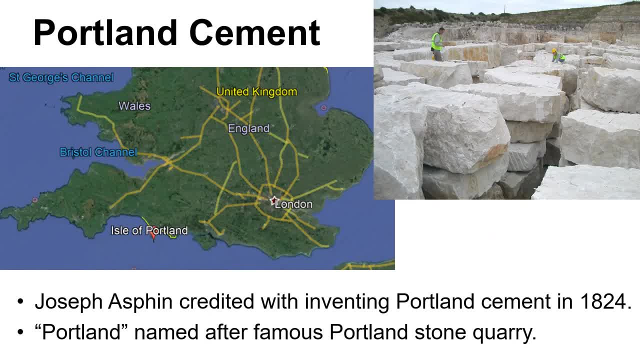 And they actually split apart And I think his son actually figured out what you know a little bit more of what actually happened, where they could actually have a Portland cement that was like a hydraulic cement that worked really well. Smedon, I don't think, did as good of a job with a hydraulic. 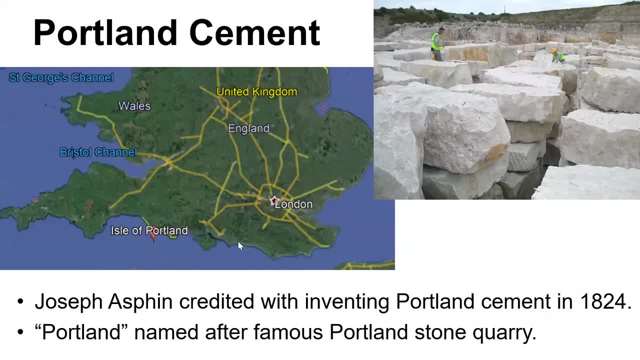 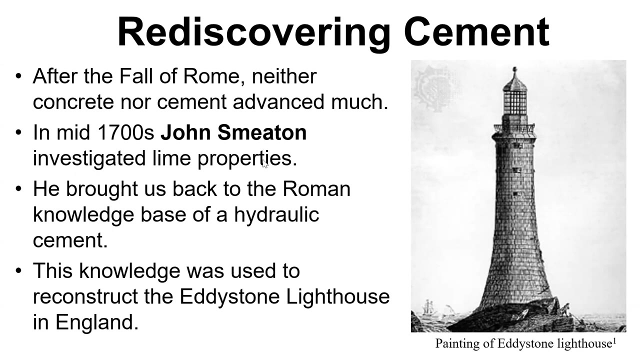 He was kind of He didn't necessarily I think he figured out a lot of that, But he was kind of at the brink of some of that knowledge. Joseph Aspen kind of came in and he really was a great marketer, So he so you know, as you had like an engineer that really dug in and tried to figure out all the different properties. 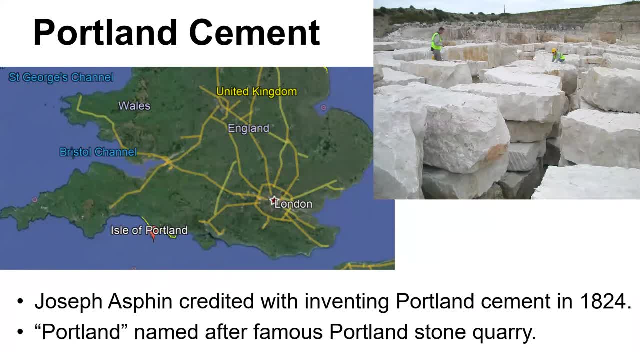 You had Joseph Aspen, who He was not not a you know What you'd think of as like a good engineer- I really understand a lot about material properties. He just kind of did a lot of trial and error and didn't really understand necessarily what he was doing. 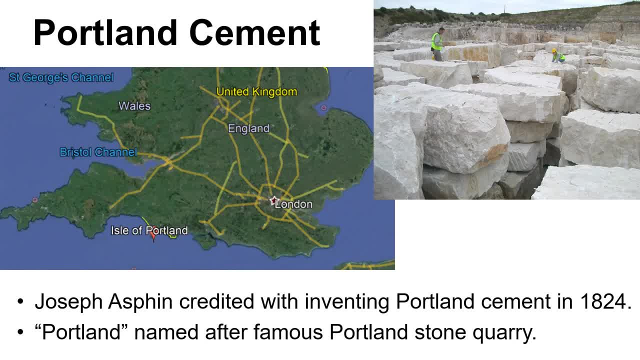 But one thing that he was really smart at was he realized that this, this cement that he was able to make. He realized very quickly that it looked. it looked like this Portland stone quarry And what was really cool about this Portland stone quarry over in England? 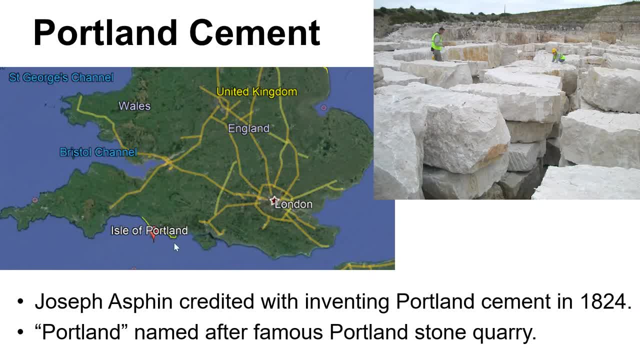 You see, over here on the Isle of Portland, They would actually quarry this stone, These big chunks of rock, like you see over here on the right, And they would take these big chunks of rock and they would put them on a ship And they'd ship them all over the world. 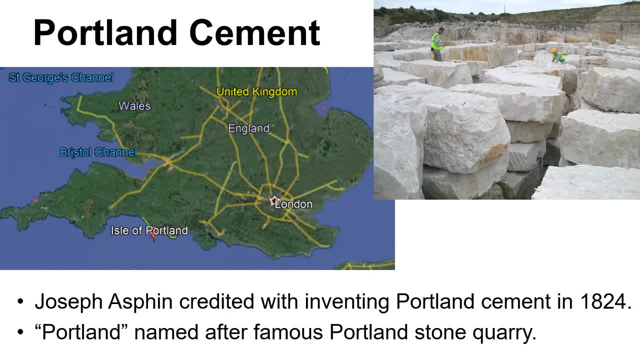 And it was kind of like prestigious- Showed you how rich you were by taking the, by having the stone, this Portland stone, And a lot of times you'd have people that would go out and chisel different stones, And it was kind of like prestigious. 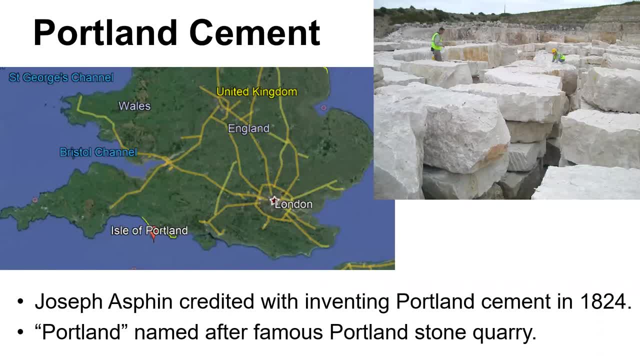 Showed you how rich you were by taking the stone, this Portland stone, And it was kind of like prestigious, And they'd go out and chisel different shapes and put all the stones together, You know, and make stuff out of them, And so they looked really rich. 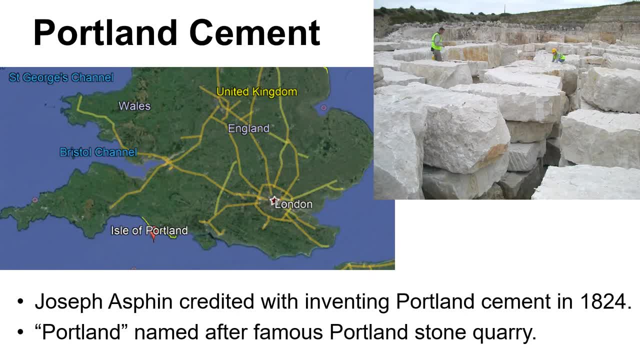 And so what? what Joseph says was: you know what this Portland cement It looks. you know, I'm going to call it Portland cement, So that you can literally take just, you know just powder. You can add some water with it, you can add some other stuff. 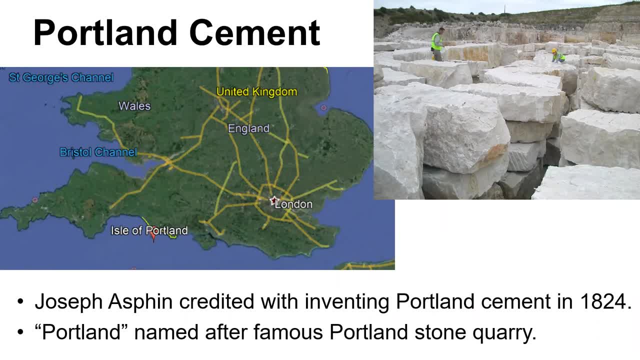 and the shapes that you want, which is a really a genius marketing. So Joseph Aspen really was a good. he had some great insight when it came to marketing. But I don't think you know necessarily he was a genius, you know, cement chemist or materials engineer or anything like that. But 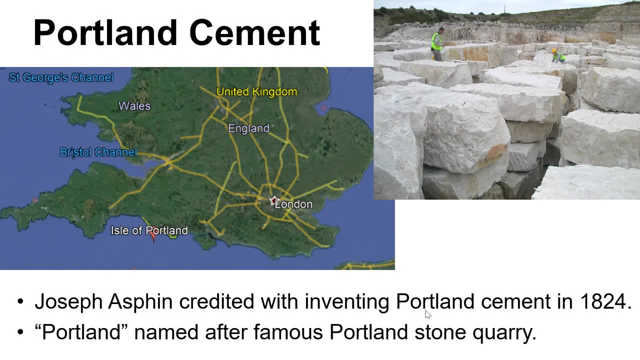 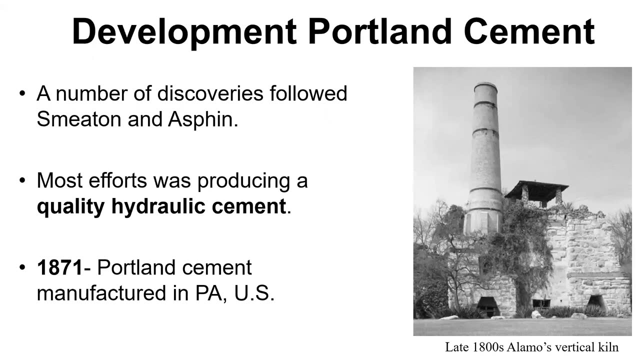 he was. you know, I think we could all say that using the name Portland was a really smart marketing tool And that's kind of how we get it. So when you hear the word Portland cement, that's where it derives from, And we'll talk more about what ASTMC 150 and what Portland cement. 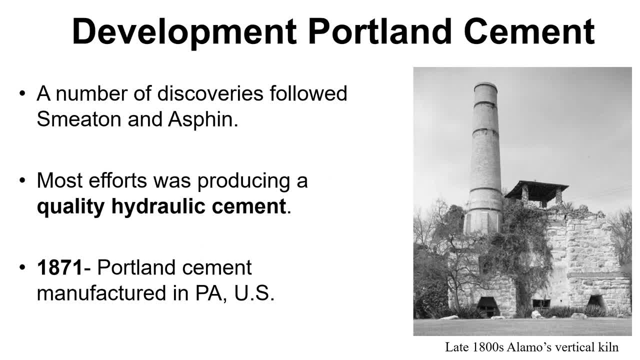 the five different types that there are coming up. So when we talk about the development of Portland cement again after Smead and Aspen, it just it really started taking off after Aspen putting in that patent And people were just like, look, I need to figure out how to make this, this Portland cement. 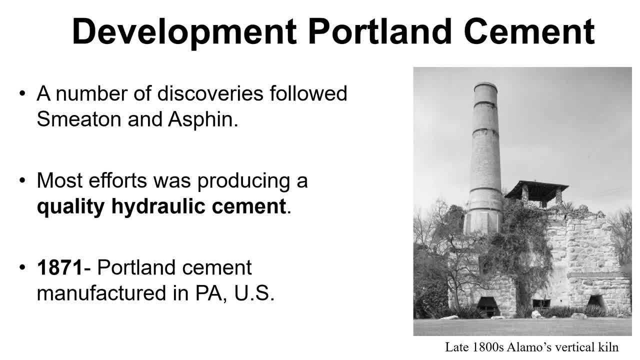 so that we can just start building structures with it, because- this is great. It is not soluble in water. we don't. we don't have any issues with the water. we just can make. you know, we can take this powder, we can mold it and make whatever stone structure. 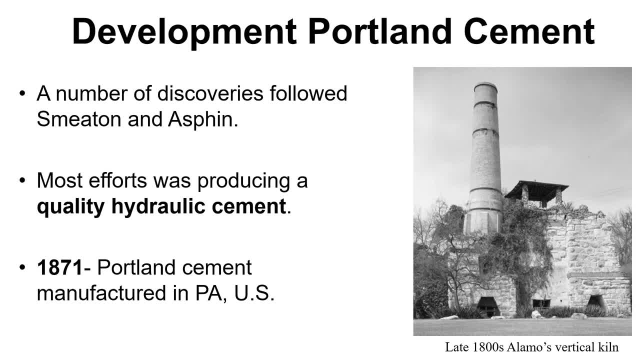 we kind of want with it. So people were just, you know, trying to figure out how to produce it the best they could. Over in Lehigh Valley, Pennsylvania, was kind of like the it place back in the 1870s. 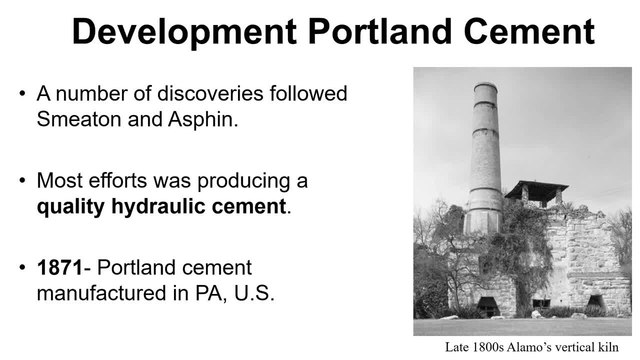 To make Portland cement. I used to work for out. I used to work for Bootsy Unisim USA, which had a the Hercules plant down Lehigh Valley. I actually took a trip down down there. It's pretty cool seeing all the different old 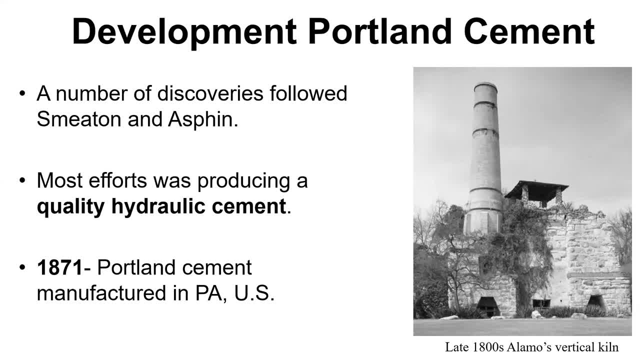 cement plants and then the ones that are still around, And there were other cement plants, like you see over here I used to work for Alamo Cement Company And over on the on the right, this is what it looked like back in the late 1880s, I believe, But this is a vertical kiln that was very, very common back then. This is: 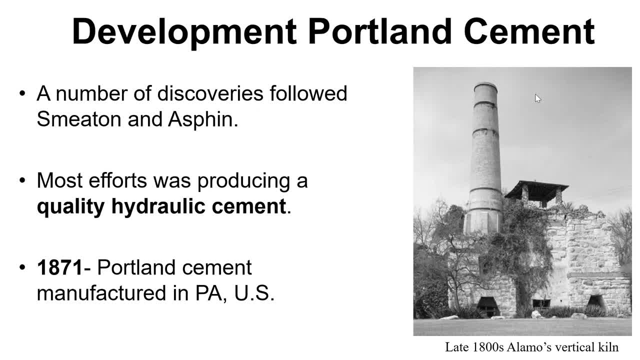 high tech And people were just producing and shipping is a wagon whatever took boat whatever it was, to ship and take in a railroad whatever and move the cement around all over the United States And in really all over the world. people were making it all over the world. 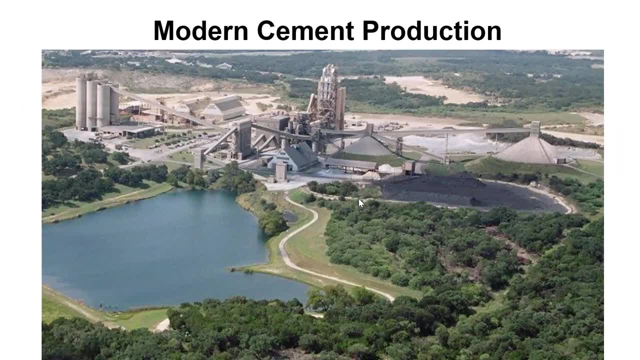 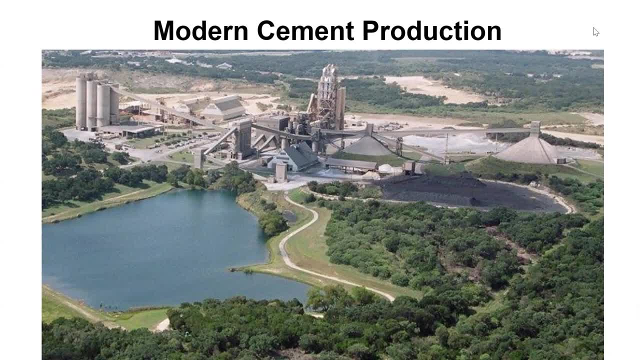 This is a modern cement plant. This is a modern day Alamo cement plant. Now this is worth over 1.2 billion with a B dollars. their electricity bill per month is over a million dollars. So you know some of these cement plants they produce, they have a high, they have a high energy demand. They do produce some CO2, I think about 2% of the world's CO2.. 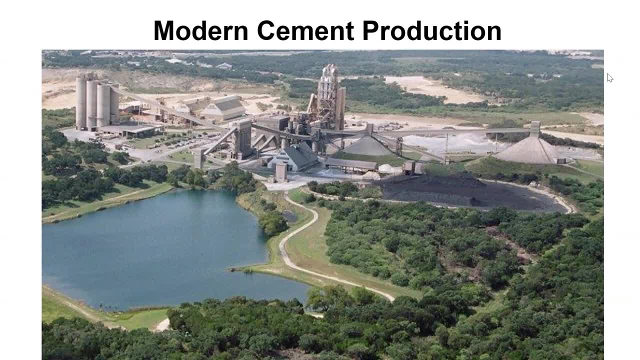 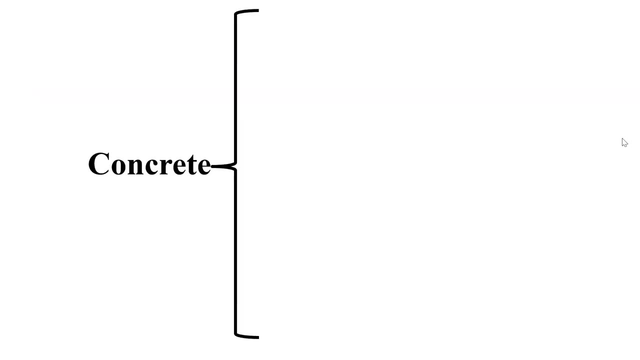 CO2 is from cement and in the world And they are a lot more energy efficient today than they even were 10 years ago. And it's very impressive how, how, how- people are developing cement, and I'll get to that in another, another lecture. 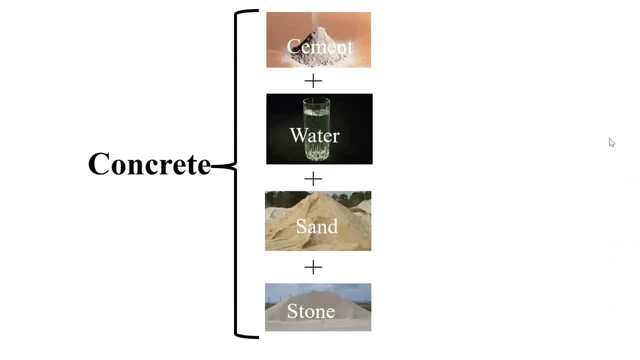 So in general, just to kind of get some basics in, concrete is made of cement, water, sand and stone. That is 19,. you know, night before 1950s, That's kind of what it was It was made out of. you had your Portland cement, you added some water, some sand, some stone, you mix it all up and it's called concrete. So in this class, when I use the word aggregate, 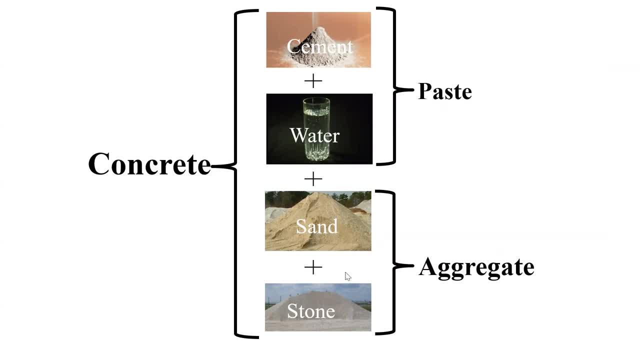 I'm talking about, you know, the sand, the stone, fine aggregate, coarse aggregate, And then for the word paste is used. That's actually talking about your cement. Maybe, if you have, you know cementitious materials like fly ash, slag. 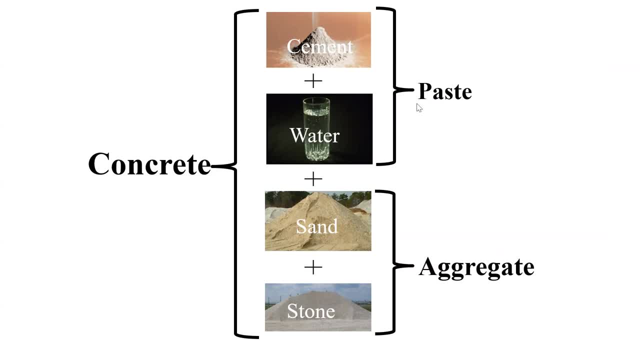 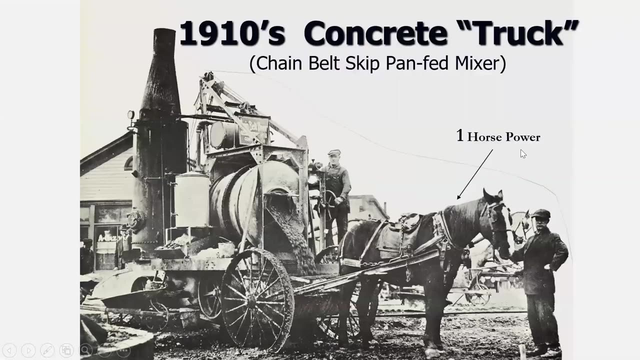 That would also be classified in the paste and water. So it has to be all the combination of cement water At least, and then you know we can add in some other cementitious materials like fly ash. Alright, So you also have. 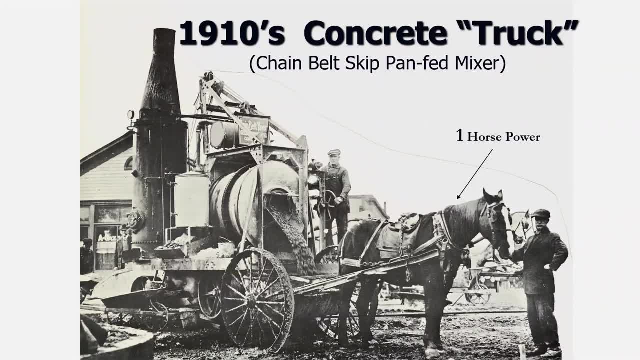 So this is a 1910 concrete truck- and I put that in parentheses Because you know this is a one horsepower concrete truck. where you may, you have your buggy. You look real close. It's this mixers on a wagon. It has its steam fed and the mixers you know, making concrete and mixing concrete together and they dump it into a wagon and they move it to you know wherever they're going to pour the concrete at. 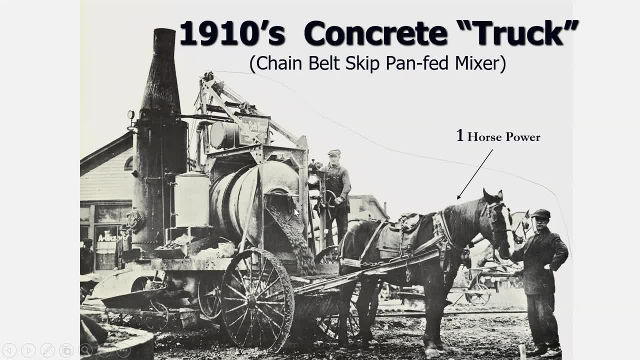 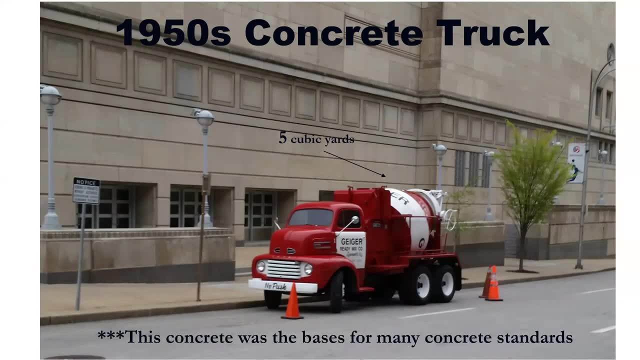 And this is, you know, one horsepower concrete truck. This is big high tech technology for 1910, And you also have the 1950s. You can move a little further. This is a five yard truck. You know, this was big time and 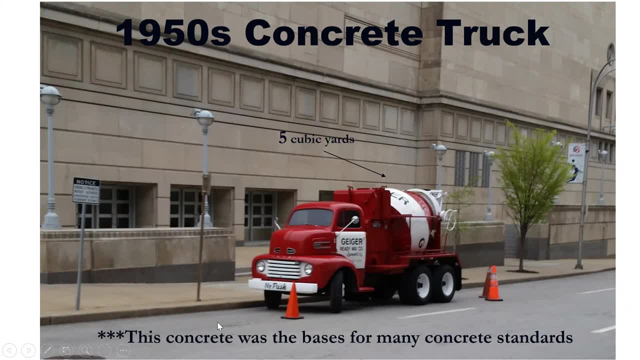 This is actually out of the ACI, out of Geiger Ready Mix. They're from Kansas City area. There's. they're good people make, make, make good concrete and But this is their five yard truck that they have And it's really cool going in and seeing it. 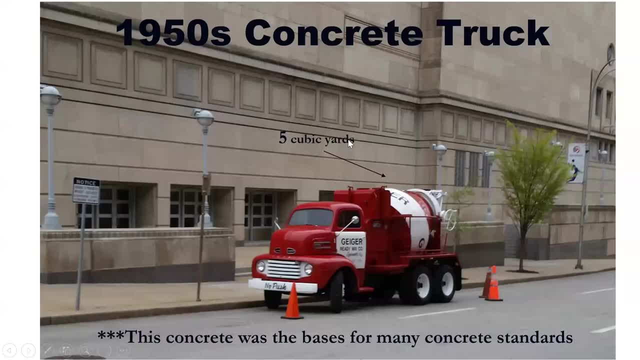 If you're ever your big concrete nerd like me and you're able to have connections where you can actually go and talk to visit their plant, that they have some really cool plants and They just have this, have a lot of really cool things going at what they're doing at their 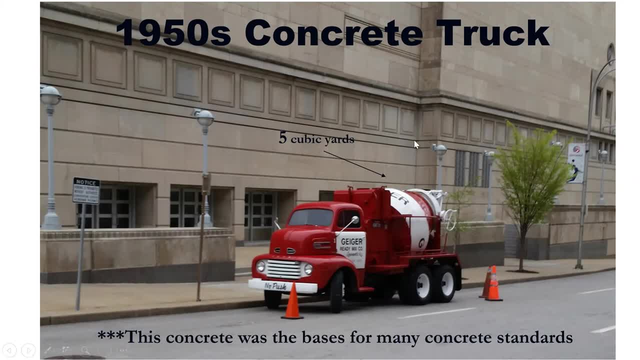 At their plants. So if you're a big concrete nerd and Europe in the Kansas City area, I'd highly suggest to check out their plants and see what they're doing. They they do enjoy talking to people that are in the concrete industry. 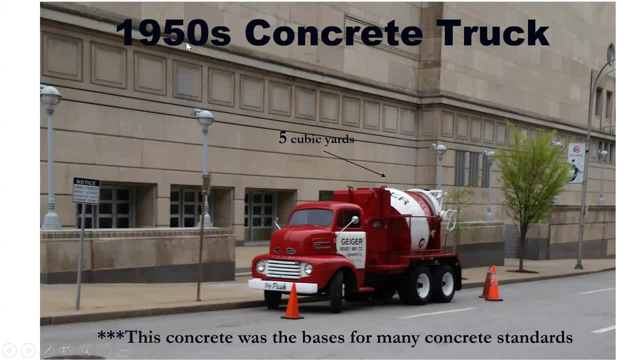 Alright. so one thing I want to kind of mention is the 1950s concrete truck. This is actually where most of your concrete standards come from. Is you know? the 30s, 40s, 50s, 60s was kind of where most of concrete standards were written, and then over the years, 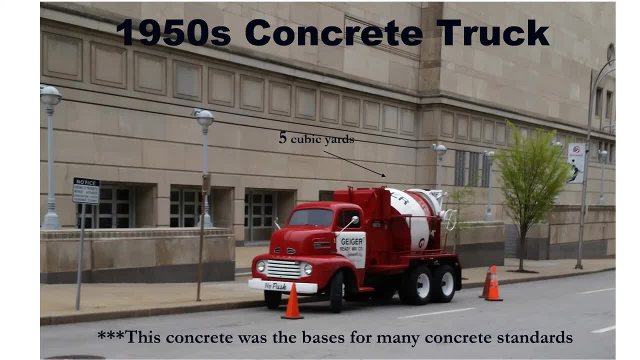 they have been evolving and tweaked and developed and and further developed, and so sometimes it's important to kind of realize where your roots were, because people don't always like change and sometimes your standards need to be rewritten because you're not dealing with a five-yard truck. 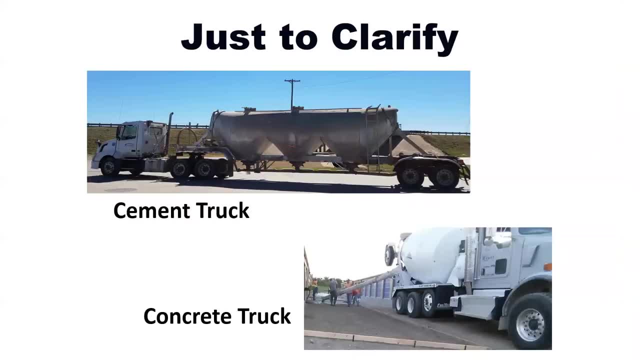 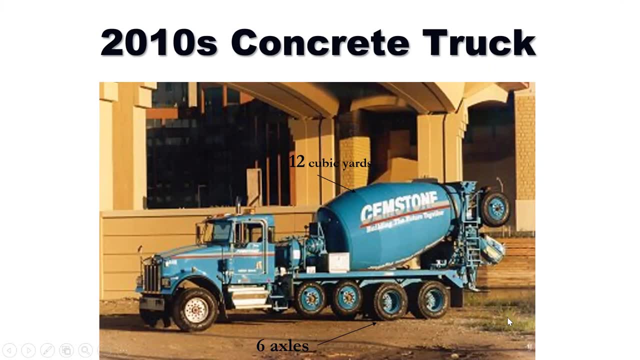 anymore. you're dealing with, you know, maybe a 12-yard truck like you see, like you see here. so this truck has six axles. this one will actually come down if there's a con, if usually if there's concrete in it, just to provide more balance and it also helps, you know, with these. 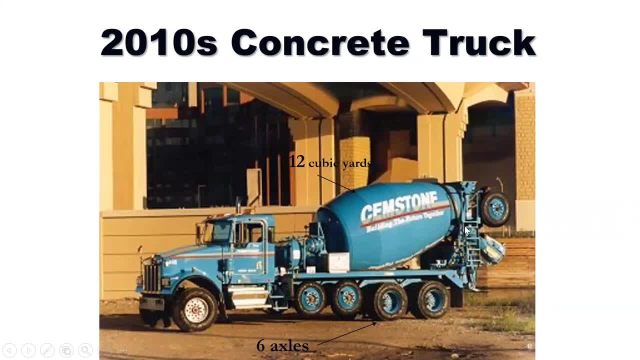 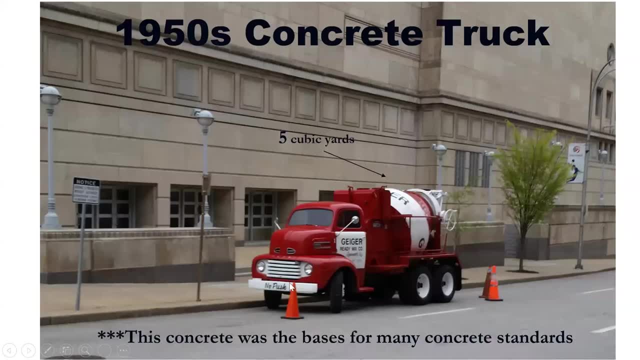 different axles. whenever the truck's really heavy, it provides more support so that it can legally drive down the road. so there's all sorts of different things. when you compare a 3 axle truck to a 6 axle truck, there's a lot, you know. there's a lot of technology. 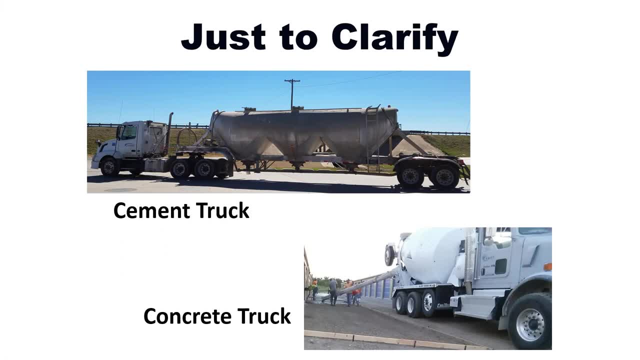 that gets changed. and just to clarify: uh, cement is the gray powder that goes into concrete. concrete's made up of, like i said, cement, water, rock sand, and the top picture here is a cement truck, the bottom picture here is a concrete truck. people get those kind of confused. 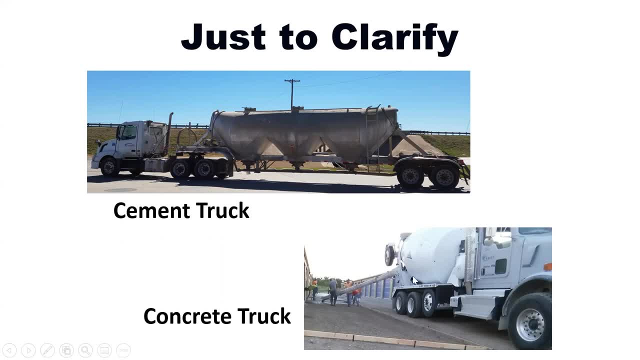 but just remember cement and concrete are different set. calling a cement sidewalks, like you know it's like, in essence, like calling a loaf of bread flour- yeah, there's flour in the bread, but that's actually not the correct term. that's just weird to call you know say: can you give me that? 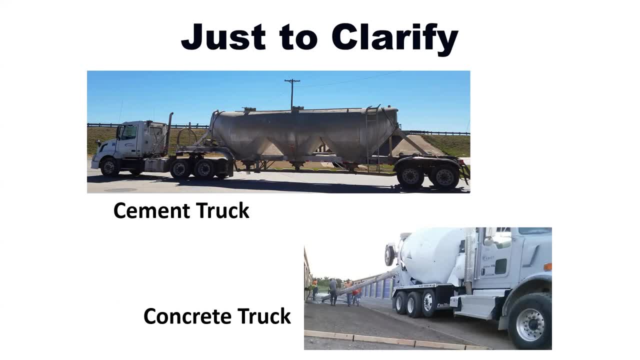 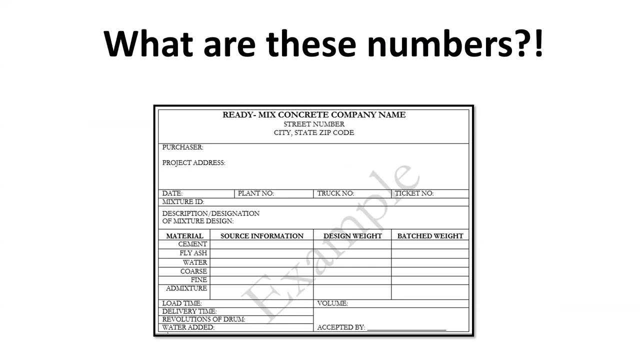 loaf of flour and people are going to look at you going, what are you talking about? there's a loaf of bread there, but not, not flour, and it's the same thing with you know, like a cement sidewalk. it's a cement sidewalk. so if you've ever went and ordered uh concrete and had it batched out and 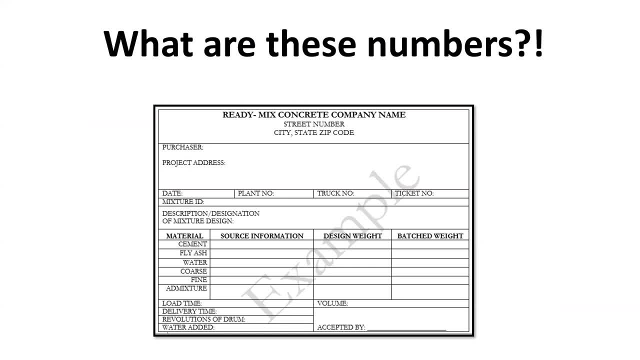 then you go and you sign the batch ticket. you look at that batch ticket and you say what the world are all these numbers? i don't get it. and you know, some of you can kind of figure it out, like the ready mix company and their address. um, you know your project address, maybe the purchaser's name? 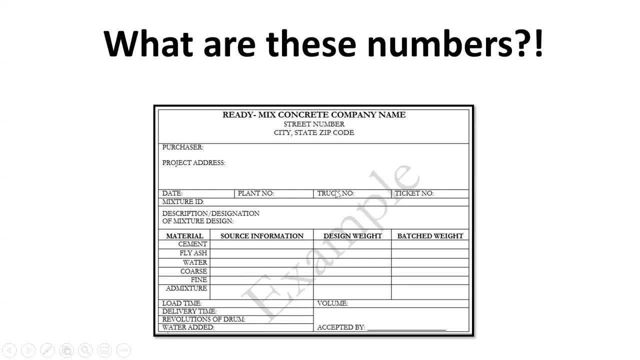 you know your name if you're purchasing it, the number of people that you're purchasing it, the number, the truck number, the ticket number or maybe the plant that that came out of. you may have some type of mixture id like 3000 psi no air. um, you know, house slab mix. 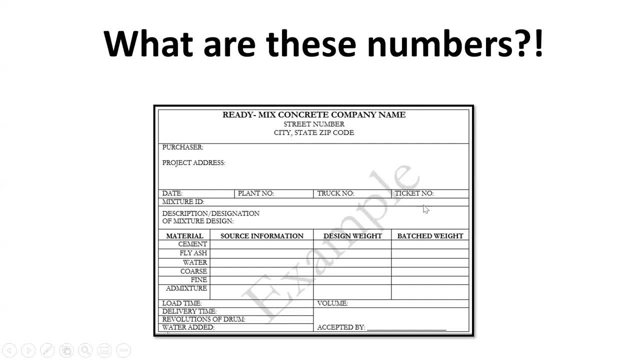 um, and you may even have a description if they need a description. down there it's very, it's pretty common- they may just have the description and the id. so instead of saying this is mix one, they may have the description in that, like i kind of said, 3000 psi, no air, no air, trained uh. 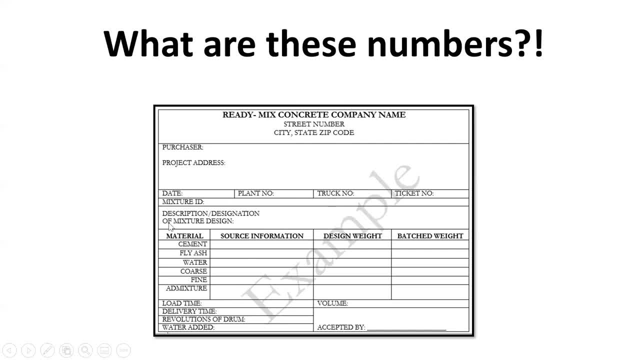 residential floor slab. you may also see the material information, mixed design information, and that's kind of what we're going to focus on- is what all that actually gets communicated. then you also have the load time, so when it was actually that concrete was loaded when it was delivered to. 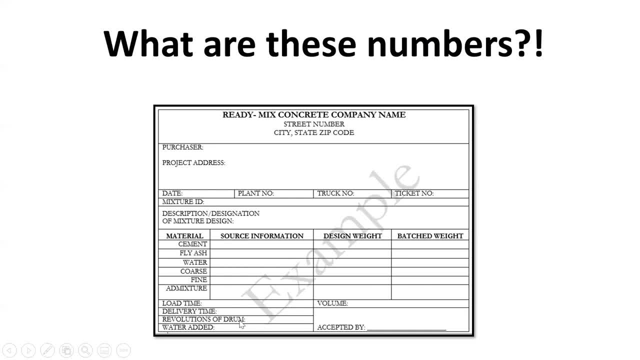 the job site, uh, the revolutions, that, how much. so how much. that drum, that ready mix truck, how many revolutions that drum turned, and then how much water was actually added to the job site. and then you may have somewhere on the batch ticket you may have, uh, volume, so the total volume. so is it a 12 yard? 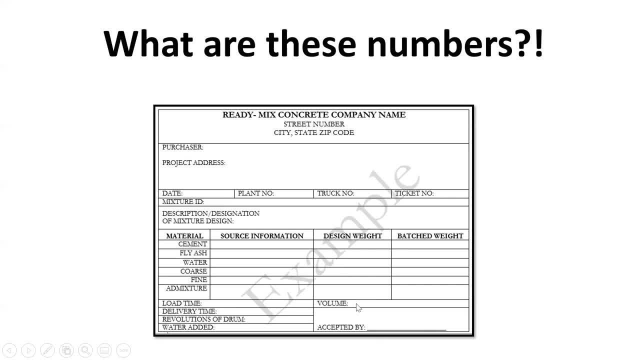 truck, 10 yard truck, uh, that's it that, sorry, 10 yards of concrete in that truck. was there 12 yards of concrete in that truck, that truck, or six, or you know a yard? i mean, where is that at? so again, this is kind of where we're. 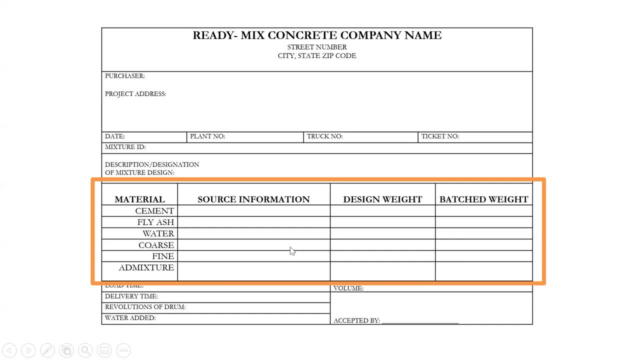 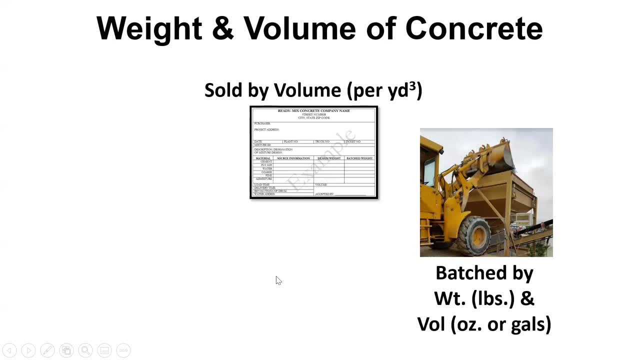 going to focus on is the materials that make up the concrete. so before we get started, when you start looking at weights and volumes on that batch ticket, you kind of get confused real quick because you really need to understand that concrete is sold by volume. so how many yards of concrete to? 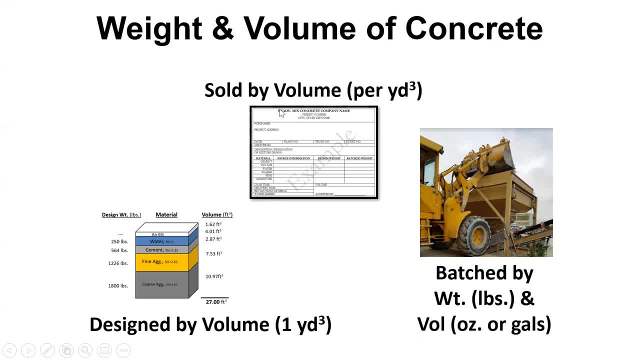 put into a, into a certain forms. so you know, you go out for a contractor, he's going to go out and he's going to measure, say he has a sidewalk. he's going to measure the thickness of of the sidewalk that he's on, that he's going to pour, and then he's going to measure the length and then the width. 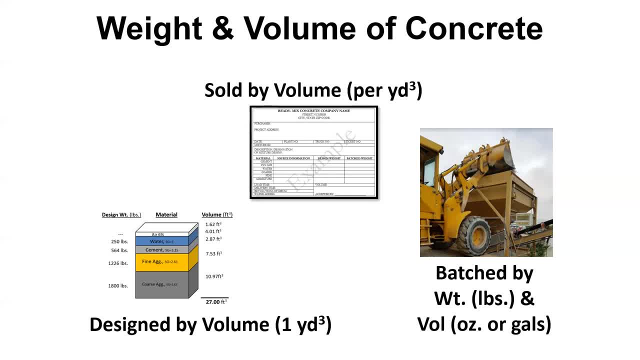 of that sidewalk and he's going to come up with a volume, um in yards. so you have to do a little conversion. you know, if you move the thickness into from inches to feet, and then you have to convert yourрос to the length and then you do a maybe Facilite around oneため. so the whole setting. 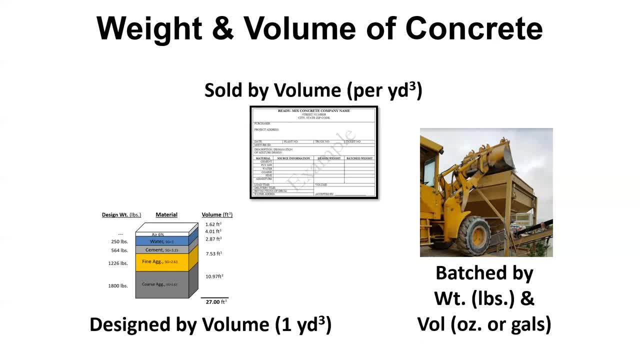 and then you have to to do a certain number of yards of concrete without measuring your gray area of daylight and so not knowing exactly how well those нам Great thanks 3 want based on a cubic yard, and then you're going to just multiply. so if you need 10 yards, you're. 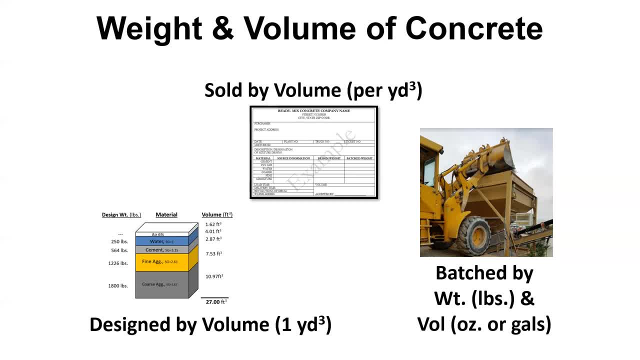 just going to multiply all your- you know, all your batch numbers by 10 to get 10 yards. so for our, for a lot of our labs, we're actually going to be dividing by 27 to to take it from a yard to cubic feet and a lot of our mixes will be, you know, 1.5 cubic feet or two cubic feet in a lab. 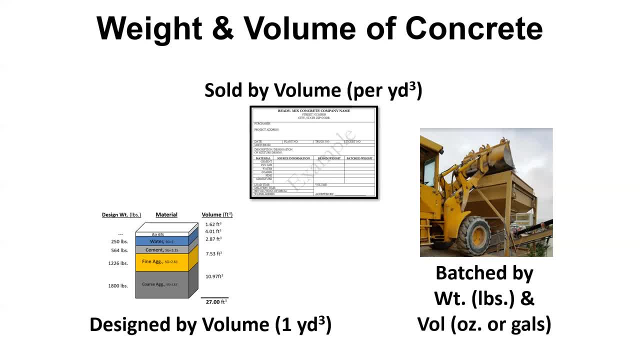 so kind of you know, recognize that and we'll go over that here here coming up whenever we need to start making concrete in the lab- then you also have the weight, volume of the concrete. so whenever you're batching- so sometimes you batch by weight, sometimes you batch by volume- typically liquids are going to be batched by volume, so you may batch. 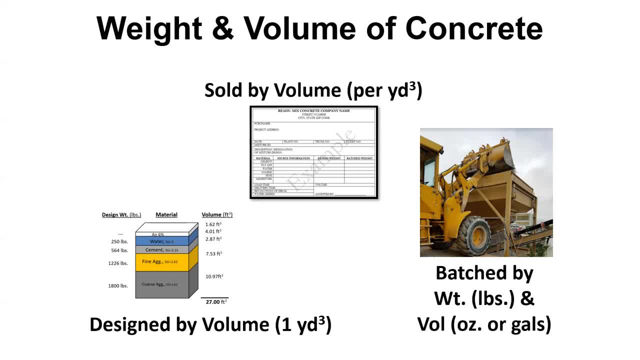 you know, say 30 gallons of water, so you may have to convert from pounds to gallons for your mix design. add mixtures: if they're in liquid form, then they're going to be. you know they're going to be a certain volume, maybe in ounces, then you have. 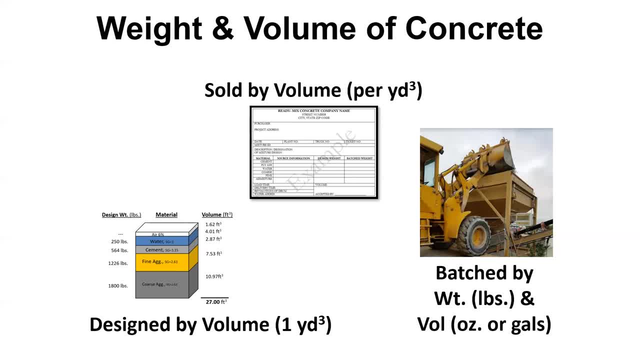 your weights, like your cement, your fly ash, your, your coarse aggregate, your fine aggregate, will all be by pounds. so you can see here this front end loader is actually dumping into a hopper with a scale that has the number right there, and then at the bottom of this hopper there's actually 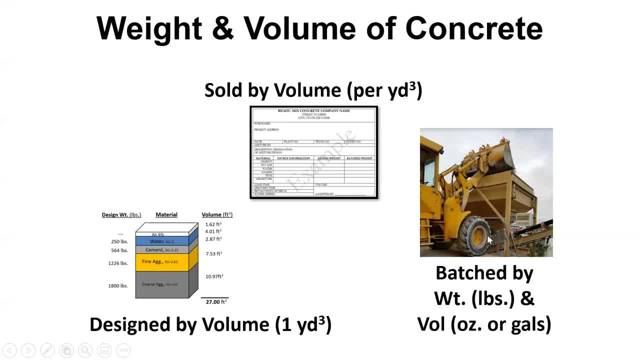 a gate with a scale attached to it. it's actually weighing out how much aggregate's going to need to be loaded. then there's a conveyor belt here to kind of take up that concrete up to to start batching it, whether it's a dry batch or a central batch. 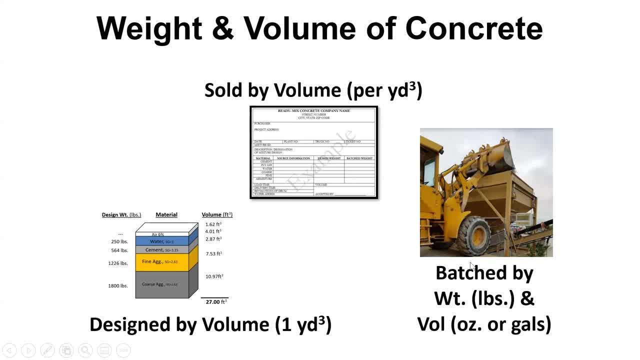 so that's kind of how you know volume and weights kind of go back and forth. they can be confusing in the beginning but there is a purpose for why you have volumes and weights on your batch tickets and they're real important to understand those differences and we'll go. 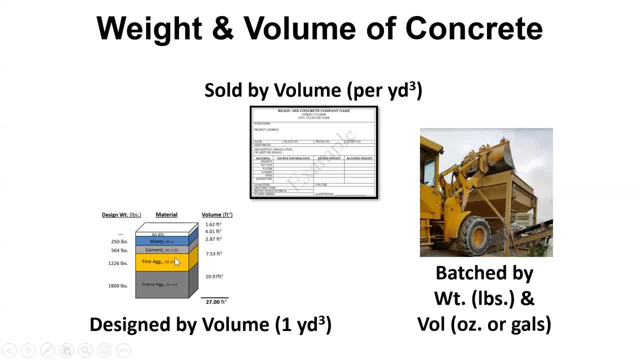 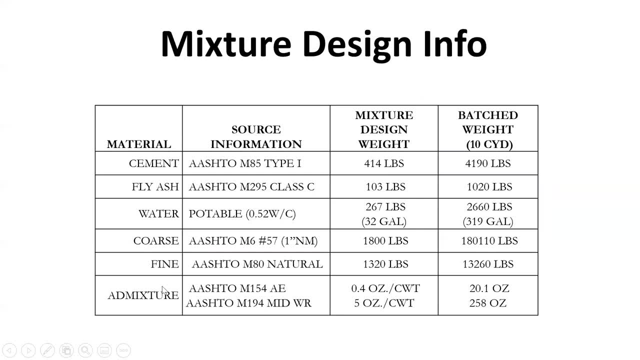 through, especially when we start talking about designing the concrete, we'll go through even more about this concept. so with a batch ticket you're going to have the material on the left and then you may have some source information. this is an ash toe. i do provide the astms also to this. it you know, tomato, tomato. 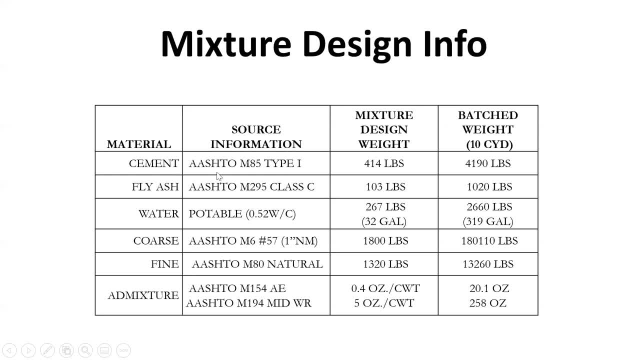 the ash, toes and the astms, the standards for the quality of material, for maybe it's for cement or fly ash or water or whatever it is. there's a standard for each of these materials and it's important to realize that and we'll go through that and coming up. 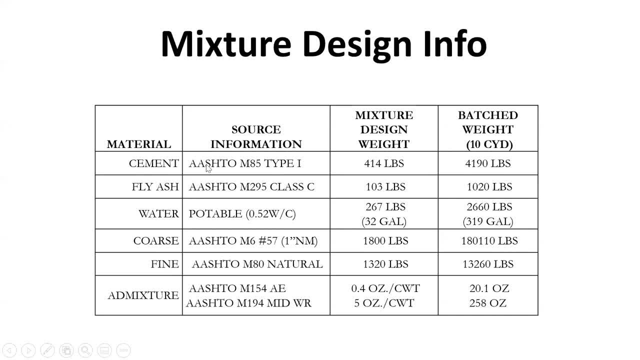 so for cement it could be astm c150 or it can be ashto m85, either one. they pretty much have the same standard. ash tow is for transportation, ashto is for transportation, ashto is for transportation, ashtm is for more of like international. it's for a little bit more of the private sector. 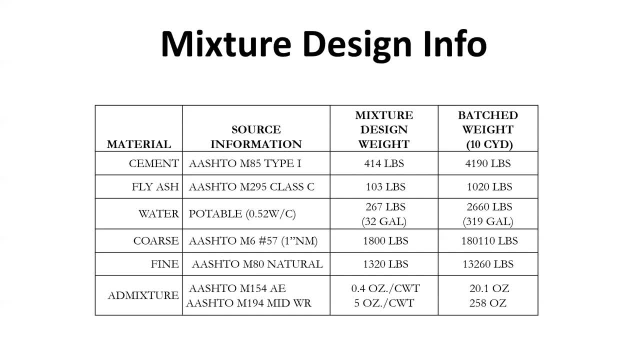 it's not just in the transportation world. so the mixture design, so how much your weight, so how much you're actually designing, is in this column and then how much you're actually going to batch, so your batch weight is over here, here so you can see, you know you have your water, which you may have 267 pounds. 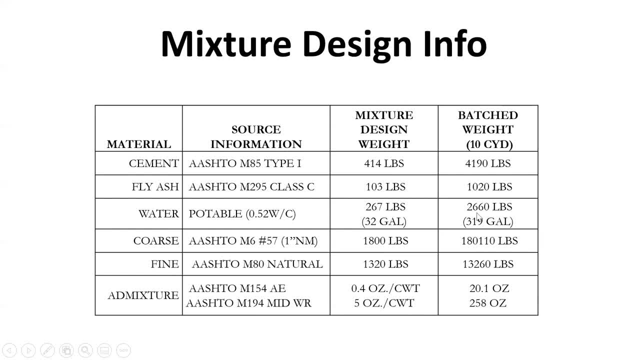 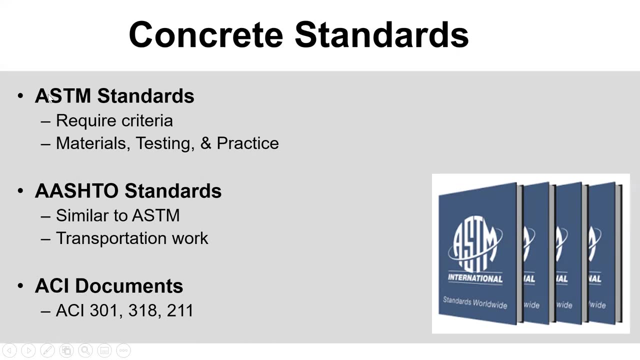 of water, or 32 gallons, and then you just multiply it by by, you know, in essence 10 to get to get these numbers. so so some of the basics. like I was communicating the concrete standards ASTM and AASHTO- again, they're very similar- going to communicate the 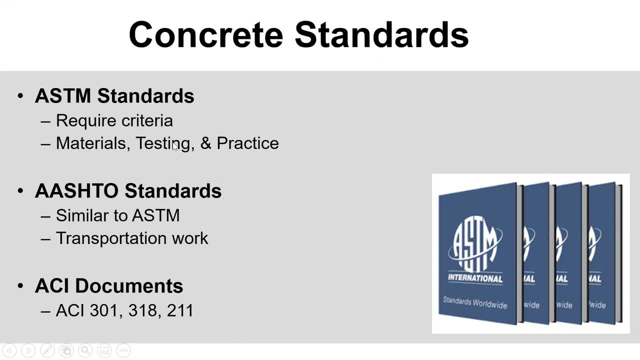 materials, the testing, the practice of how to do something. so, whether it's a, you know, there's a standard for aggregates. there's a standard for ready mix concrete, cement, flash, whatever it is, there's a standard for it. there's also a standard way that you're supposed to test. 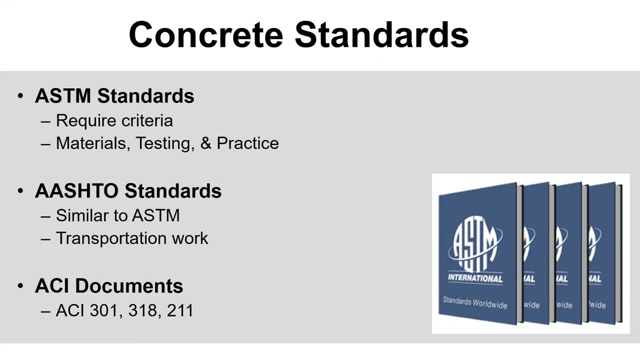 to conduct a test, so there's a standard way so that you don't have less test variability. and then there's also like practices, so things like how to go out and sample, you know, concrete or aggregates. there there's a practice, and it's also important to kind of realize that ASTMs are not just in the 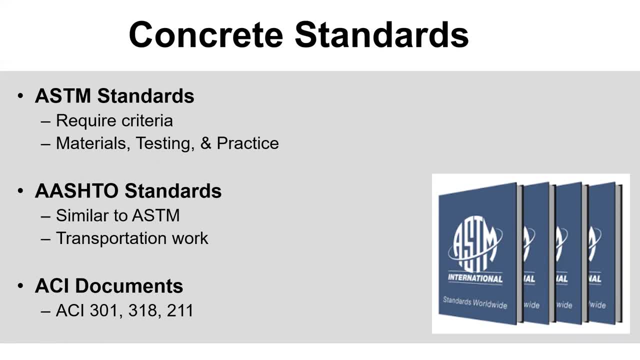 construction industry. but I mean, I think you can even find an ASTM on how to push a broom, how to sweep properly. I've seen them on the back of ketchup packets- everyone. I've seen them on the back of ketchup packets everyone- once in a while. so you know that it's ASTM, is a, you know, is more international and it's a lot more. 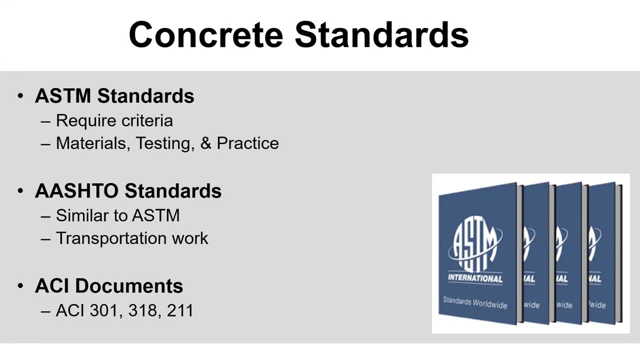 broad. AASHTO is just for transportation work. really all the state DOTs come together and they develop standards. I've actually wrote AASHTO standards and then had a DOT committee with DOT members on it actually go and submit it and go through it and see if it works and if it doesn't. 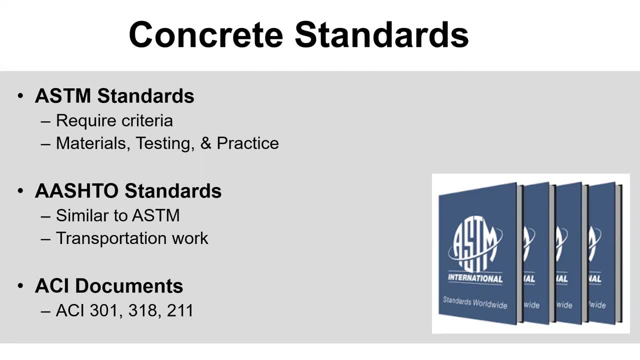 and go through the whole process and approve my standard that I wrote so. so it's pretty cool to see that process and how and how it unfolds. ASTM: they have a very similar one where they have committees, just like AASHTO, but their committees are a little bit more, they're not just 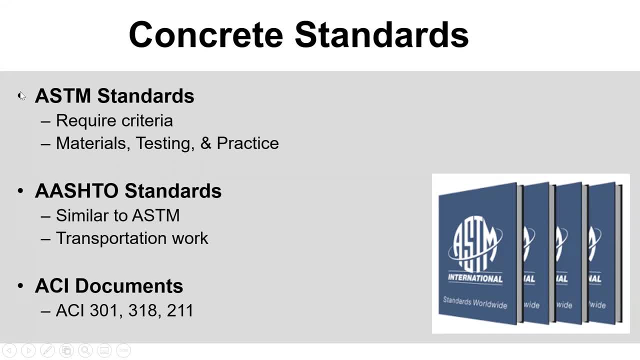 transportation, but they're kind of a little bit of everybody and they try to make it where it's a really good blend. I used to be on some of the committees for a the entire sitting on the committee with me and going to committee telephone calls. they say: 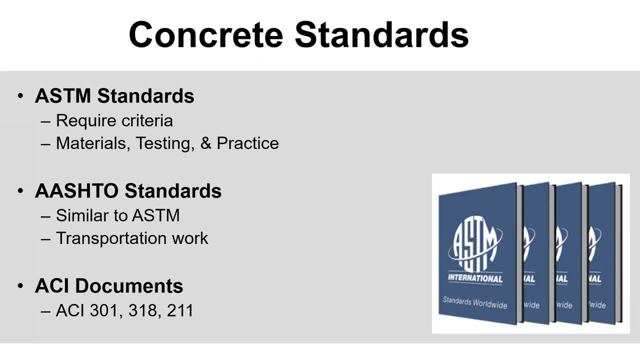 okay, what's your name? you know what they're doing and I don't know why. well, a question I came up with myself. I think that being on meetings just right quickly became dreams. so, girl, I was thinking, this year, I think, the service will start to really help me learn more about those. 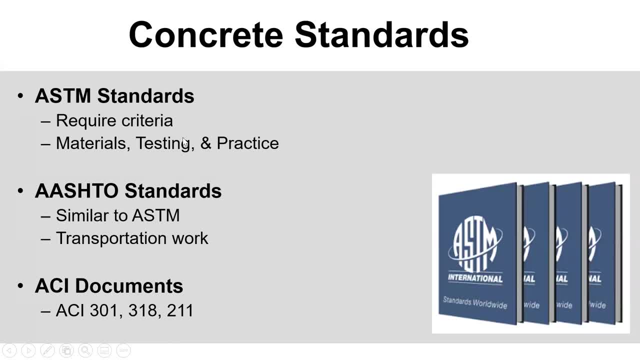 strategies and what they're doing and just telling me to actually keep in perspective what the things that we think about their culture is okay". and so again we're covering all internally, like it just happened before, the standards. so some of them were very creative and how they were trying to. 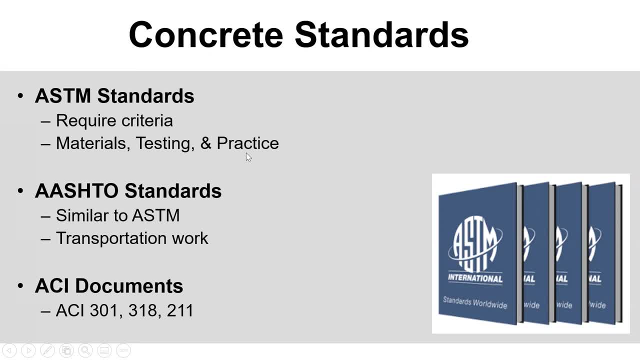 reward stuff so that it was it made more sense for today, or maybe a technology change stuff like that you also have in general. you have ACI, so American Concrete Institute is an international global organization that produces documents. I'm actually on ACI 302- construction of floor slabs- ACI 211. 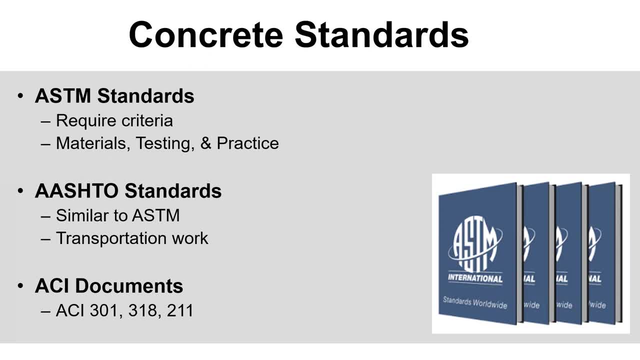 which is mixture proportioning of concrete. and then I'm also on ACI 309, consolidation of concrete. in each of these committees I named off three that I'm on, but there are there's for sure over 50- I forget how many- off the top of. 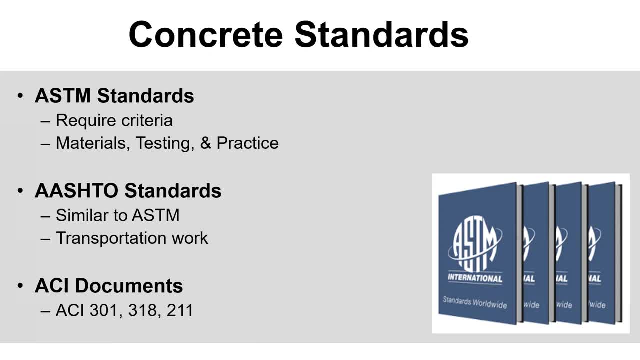 my head committees that are. you know, in essence, there are people that are specialized in certain parts of concrete. believe it or not, there are well over 50 different committees that are that are specialized in in different parts of concrete. so you think that concrete is pretty basic, but it's really not. it can be pretty complex. 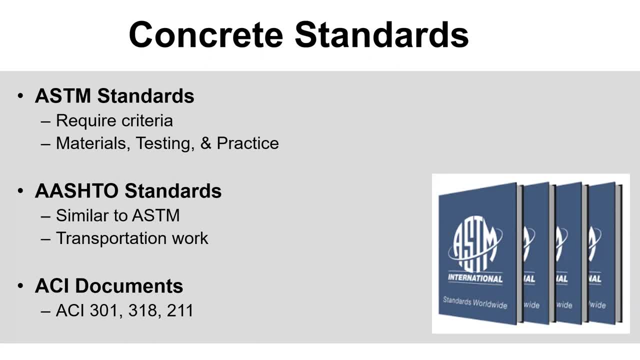 and there's a lot of good specifications and guides and other things out there: ACI more on building codes and stuff like that, like 318 301 or specifications for for concrete, for for building concrete, and some of these other ASTM AASHTO they're. 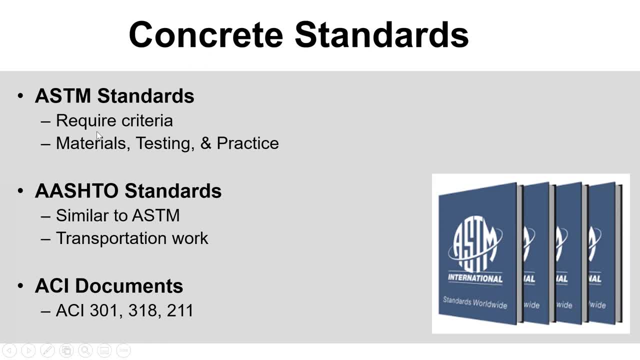 not you know building codes necessarily, but they're more of the standards for the materials or the testing or the practice. so ACI a lot of times will reference and say, hey, you need this type of cement or this type of aggregate to meet these. you know this ASTM or this AASHTO specification, so just kind of be. 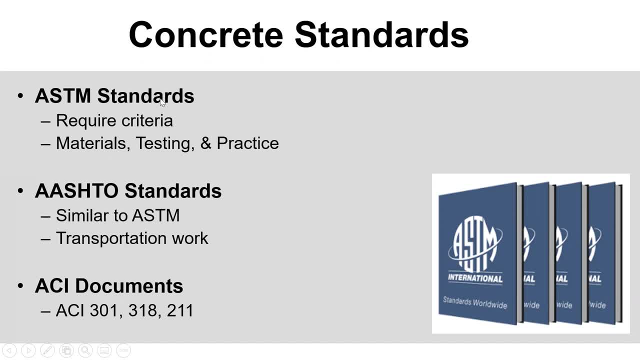 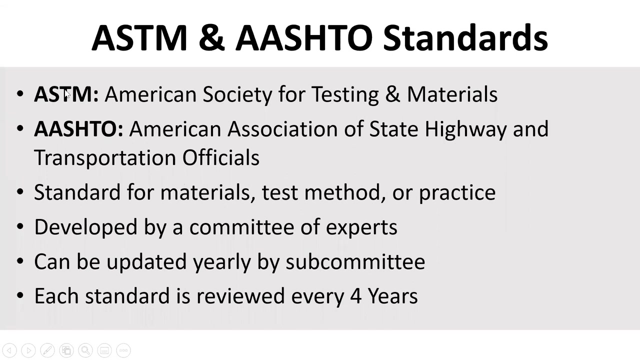 aware. so ACI is more of an engineering thing and then ASTM and AASHTO are more of you can even think of it more of like a materials engineering, more of a supplier and testing testing company type standards. so there's some pretty big differences. so ASTM is the American Society for Testing and Materials AASHTO has 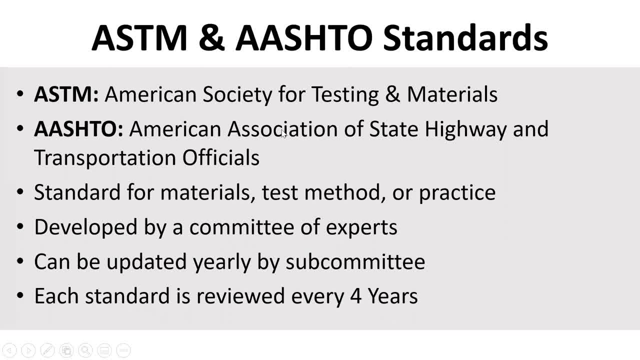 changed a little with their name, but it's currently it's the American Association of State Highway and Transportation Officials. one thing I probably didn't already mention was that you know, the standards are usually updated yearly. some of them are just grammar errors, some of them are a little bit bigger. it just depends. 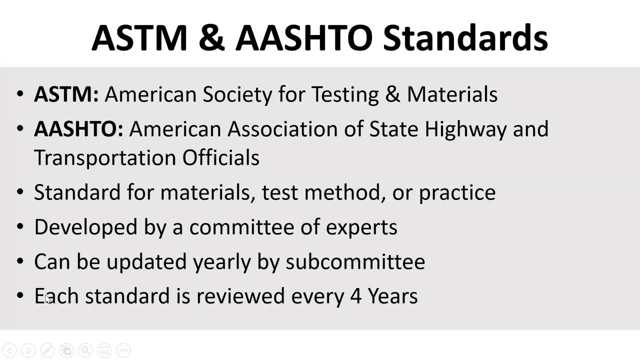 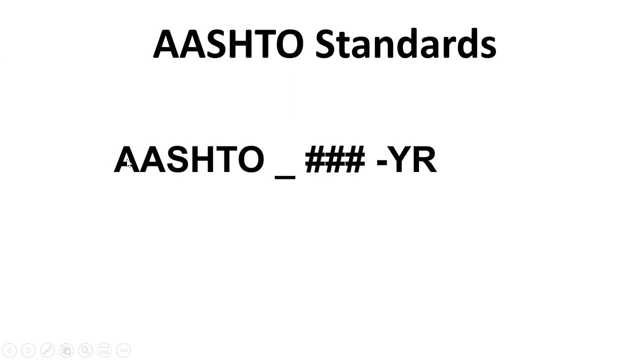 on what you're talking about. each of the standard is reviewed every four years. so you have to have a good, thorough review every four years by the committee. so whenever you look at AASHTO standards, you're going to see AASHTO and then there's going to be a blank and then a 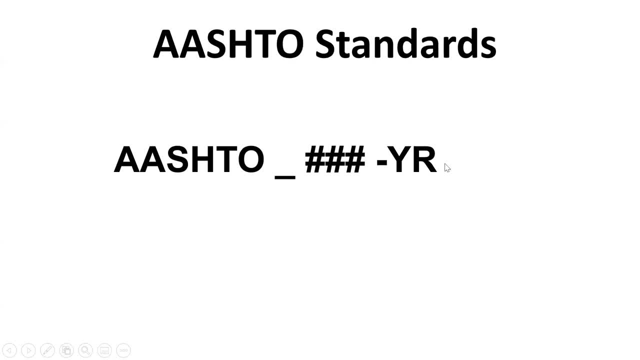 bunch of numbers and then dash a year. maybe there may be a year behind that, so you may have AASHTO, and then right behind that you're going to have a letter. so M's for the material specification, T's for the testing standard, R is actually for practice. 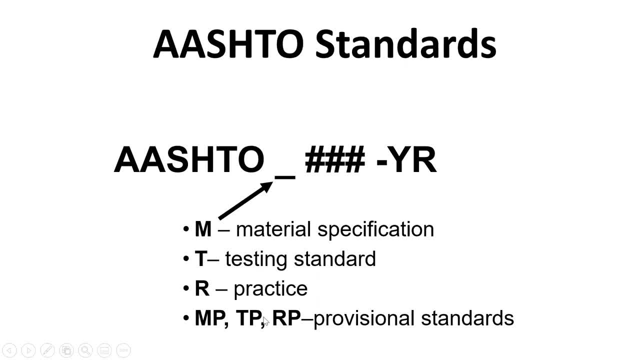 and then if you have say, like an MP or TP and RP, those are actually provisional standards, meaning we just wrote a standard and the standard may actually change some. it's temporary, really, we're going to just test it out, and so it may change quite a bit over the first few years. just to kind of 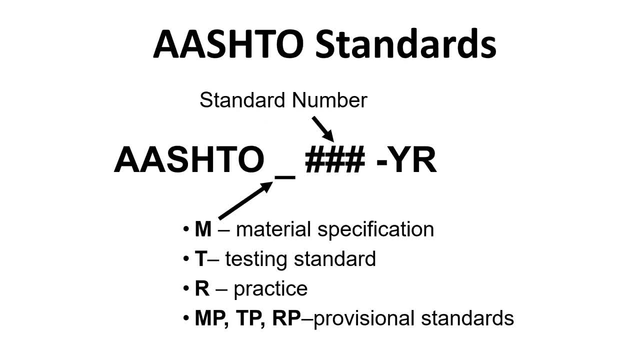 make sure the standard makes sense. and then, right after that that letter or two letters, you're going to have a standard number. that standard number is whatever that committee assigns to it. so it could be, you know, if it's 80, you know if it's M85, for 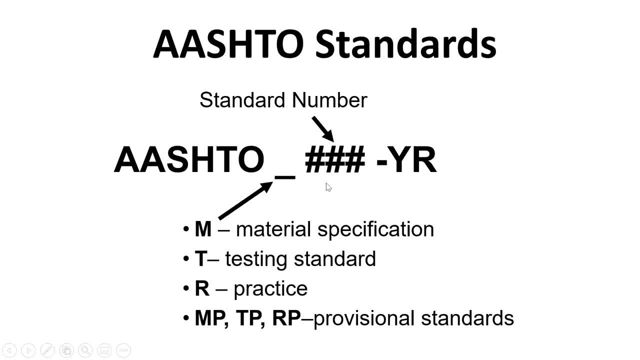 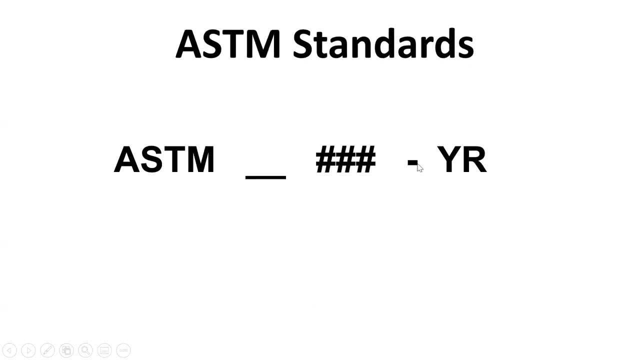 cement that 85. it was just bought ashto and the ashto committee. it's just the number that was provided and then if you see a dash and say it's, you know, 20, then that's the year that it was published, so 2020.. with astm they do their stuff kind of similar. um. the very first letter is: 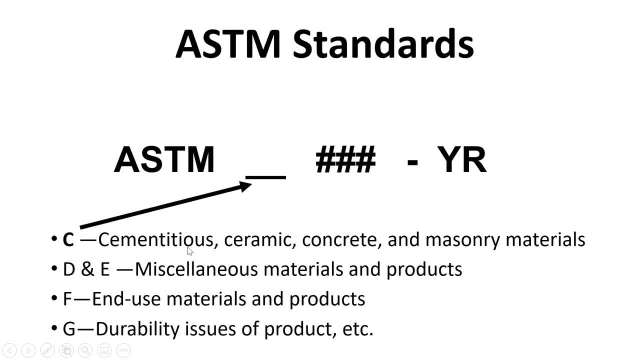 actually all times you're going to see a c for cementitious, ceramic, concrete, masonry type materials. sometimes you'll see like a d on some of the stuff because it's kind of miscellaneous materials or products. so sometimes you'll see for a practice you might see a d. 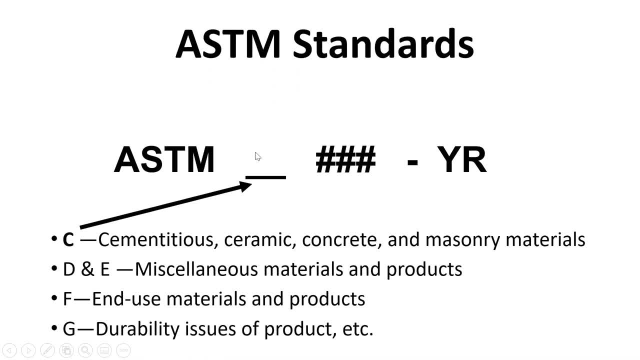 every once in a while, but most of it's going to be a, c and then, right after that, again, just like ashto, the a stm. they're going to have a standard. it's whatever that standard number it is. so astmc 150 is, you know, the standard for portland cement, um, and that 150 is just what was given. 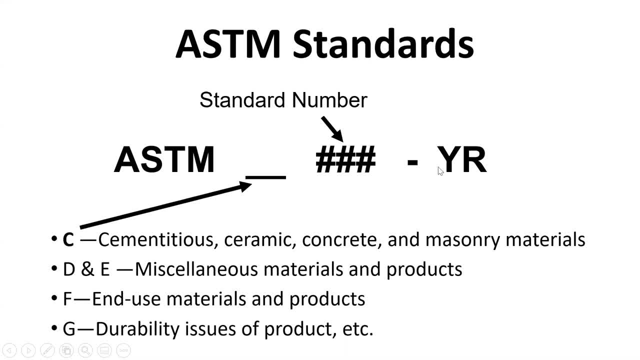 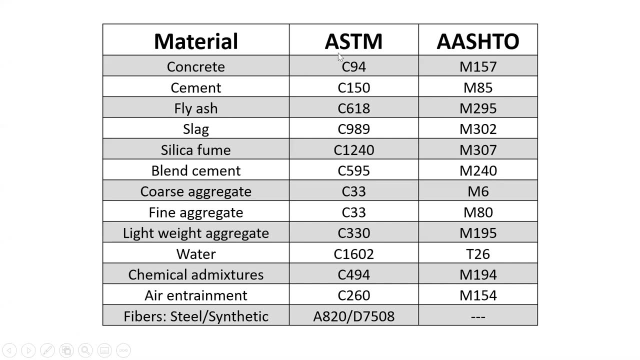 from the committee. then you're going to see a dash and, just like ashto, there's going to be a year. so if it's 20, it's, you know, year 2020. if it says 15, it's year 2015.. so to kind of help the confusion between astm and ashto, i put together this table. 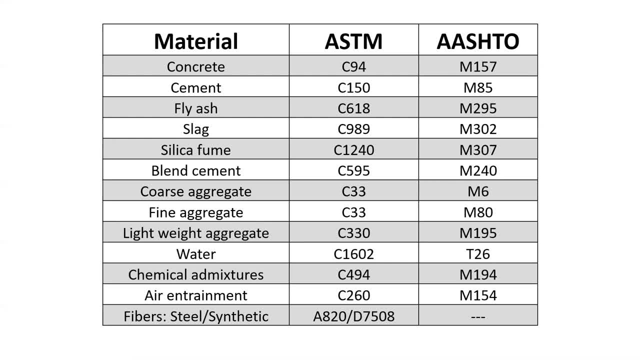 a few years back they actually had a big court case where that where people were saying they couldn't merge because they were trying to merge these standards kind of together where they wanted to be separate organizations but but just use the same standard because there's so much redundancy and the courts communicated that they could not, so now they've. 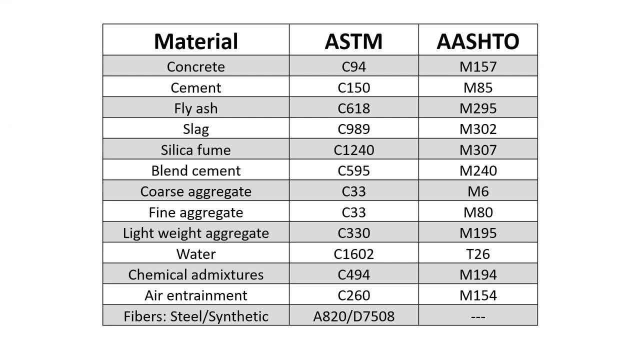 kind of backed away and astm or ashto have been making their own standards from that. so just kind of be kind of recognize that all right. so this is kind of a good table to kind of help for just materials in general, for concrete and aggregates, so you can kind of see what the astm is or the ashto for it. 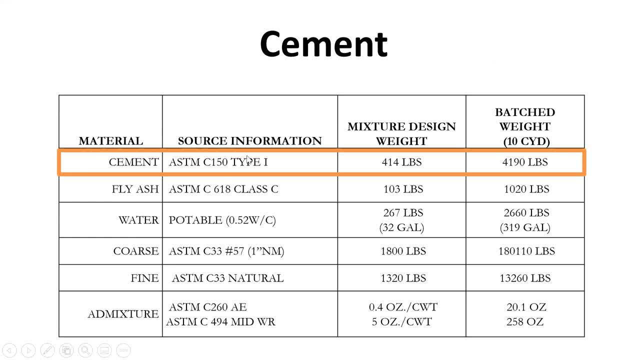 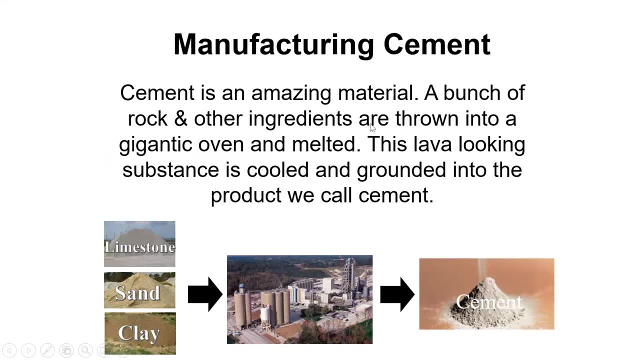 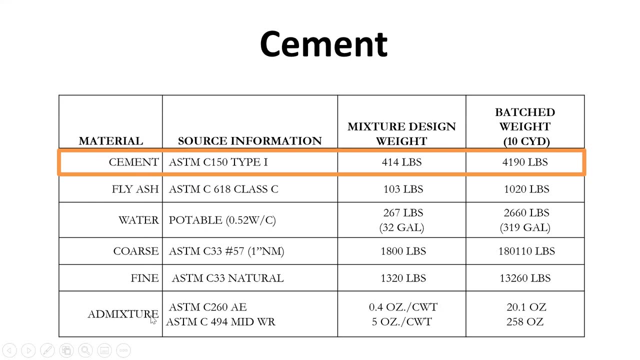 and so for cement. let's go to the next slide. let's kind of talk about cement for a minute. so basics of cement. we'll go through. i should say before i start: we'll go through each of these materials in an individual lecture. so we'll have a lecture over cement. we'll have a lecture over 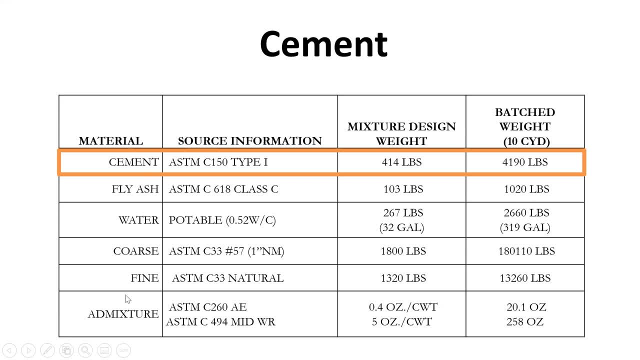 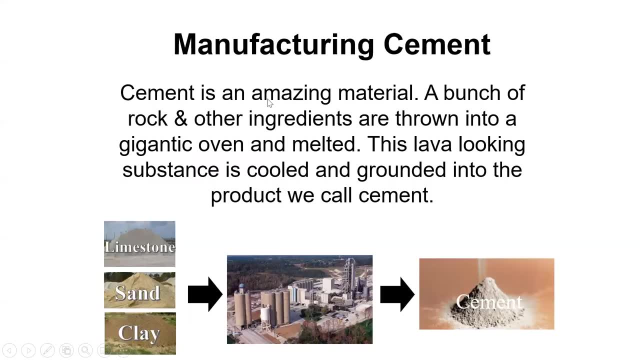 fly ash. a lecture over water, a lecture over coarse aggregate, a lecture over fine aggregate and, that's right, a lecture over add mixtures. so, um, just kind of the basics about cement. is that gray powder that goes into concrete? you pretty much you take a bunch of 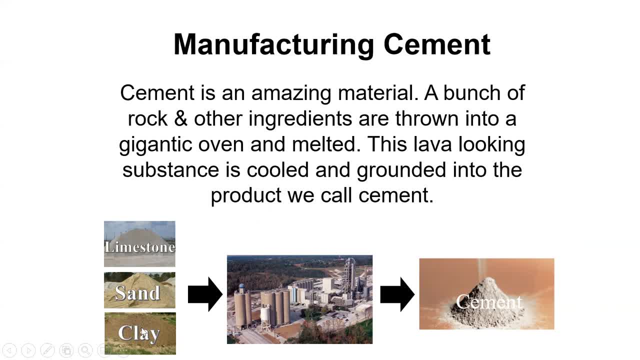 uh, limestone, sand and clay. you put it into this gigantic oven called a kiln and melts down into until, in essence, uh, lava. so it's like a man-made volcano inside this gigantic oven, gigantic kiln. that's really really hot- 2700 degrees- and eventually, by the by the end of it, it actually cools down. 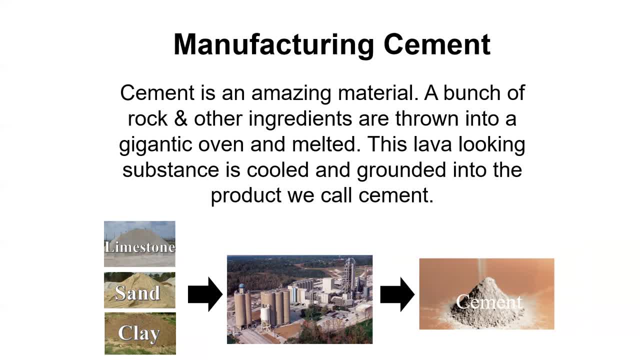 this oven again turns in a certain way, at a certain slope, and by the end of it, by the end of your clinker- cooler that- that uh looks like little bitty clinker balls is what they're called, and this little gray spherical ball can be actually ground up into cement. 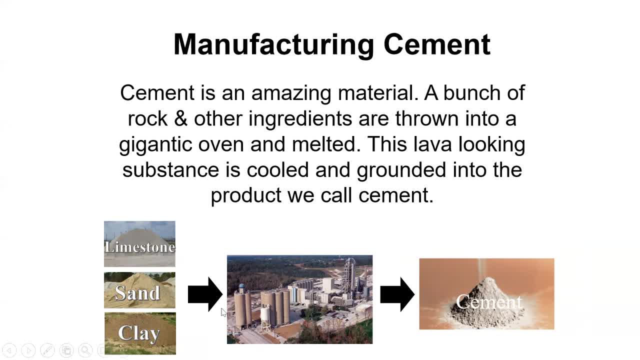 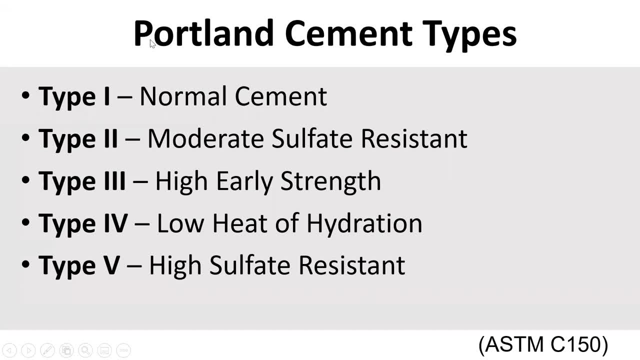 so it's really cool. um, you know how it gets put through this plant and it makes cement. we'll talk about how that kind of works here in a little bit. so we talk portland cements. there are five different types in general. type one and type two are the most commonly used cements in the united 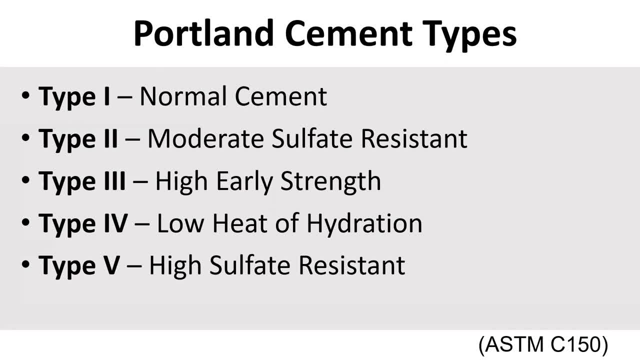 states a type one two is probably um the product that i see most commonly used in the united states, which is, which really is a type two cement that that meets the standards for type one. um, so a lot, of, a lot of engineering standards will say: for this project, i need a type one. 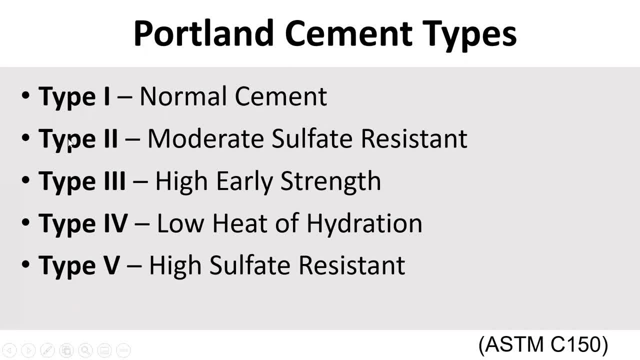 cement. well, they really produce a type two cement and a type one cement. the cement meets both standards. so those put type one dash two um. so it's really common in the in a lot of the difference between a type one and a type two deals with the c3a content um, the c3a in cement. 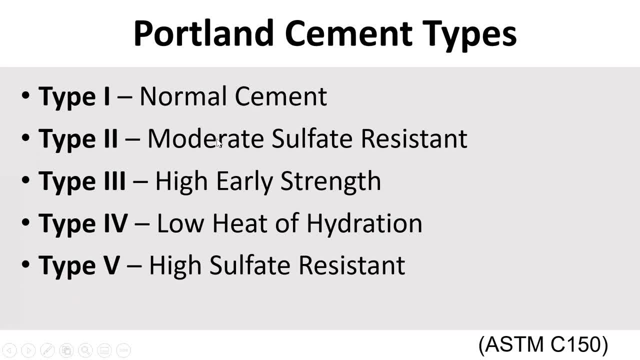 can actually um, you need to re, you reduce it. so if it's above eight percent um, it's a type one. if it's, if it's between five and eight, it's going to be a type two cement. and then if it's below five percent, if it's. 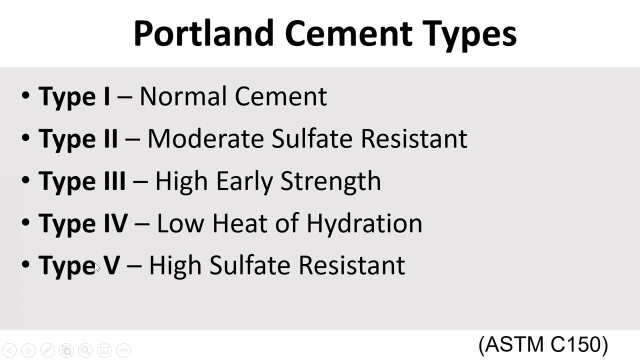 five percent or below, then it can be a type five cement and this and this three c3a actually can react with sulfates, like if they're in your soils and cause sulfate attack where you have cracking and and, uh, erosion of of the concrete. so it's 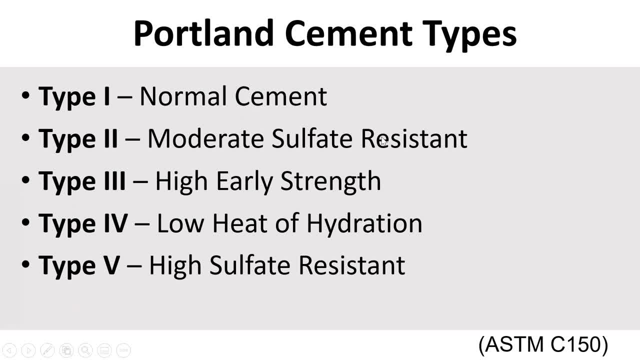 not a good thing to um if you have sulfates in your soils. now, c3a is a. you know there's a lot of great things, a lot of great attributes about it with strength and setting time and such and um, but you just got to be. 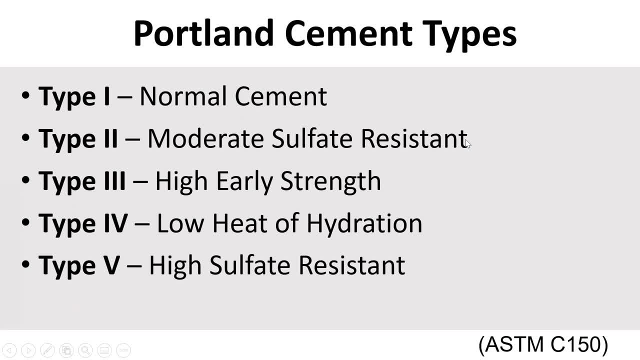 you know, got to be kind of realize that if you have sulfates in your soil, you you may be asked to have a type two cement, um, type three cement, what that is, it's high early age strength, so it's usually a type one or type two cement. 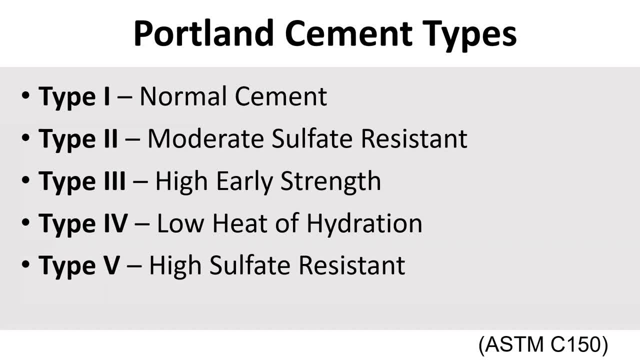 and they just grind it even finer so they have more surface area, it reacts faster and you can get those high early strengths up front. but you know what. what you know what the negative is is you're not going to get as high strength as you get your plastics further on down the road. 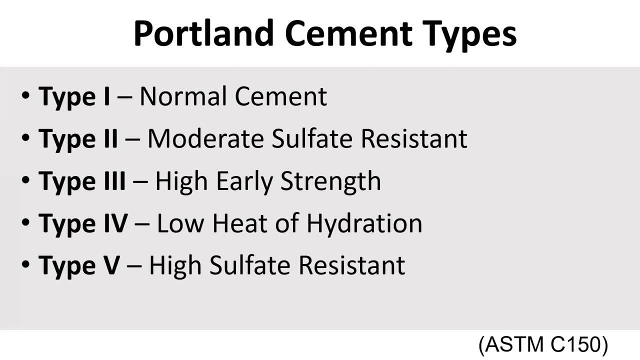 type four cement, a low heat of hydration that's actually made. it was built for uh, for the huver dam. that's the reason why type four cement was developed. they really didn't use it a lot on other on other projects after that, and so now you can just really use a. 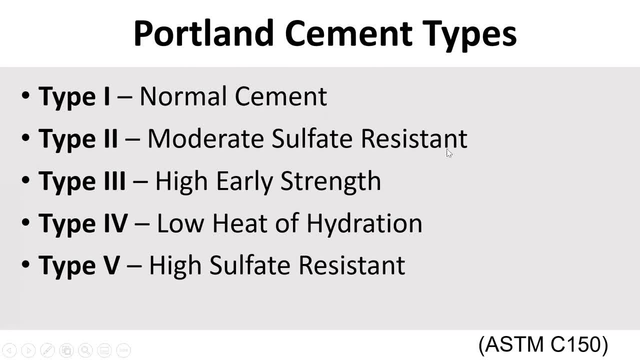 type 2 cement with um fly ash replacement, so class of fly ash at usually at 25, and then the c3a rieps. the type two cement with an 30% replacement usually does a pretty good job of low heat, of hydration. I should also point out, with a type 5 cement right here, the high sulfate. 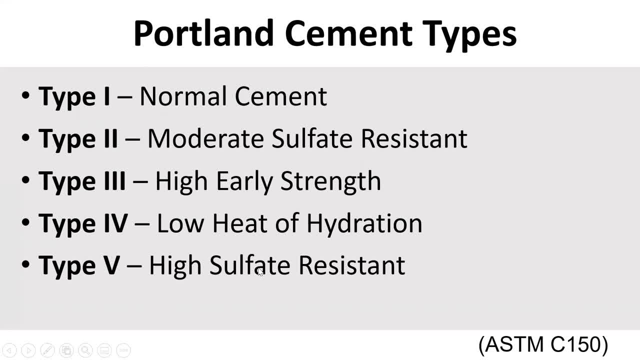 resistant that there's probably, I believe, eight plants the United States that actually make a type, that can make a type 5. a lot of them don't, and out of those eight I think maybe three have made a type 5 in the last five years. so 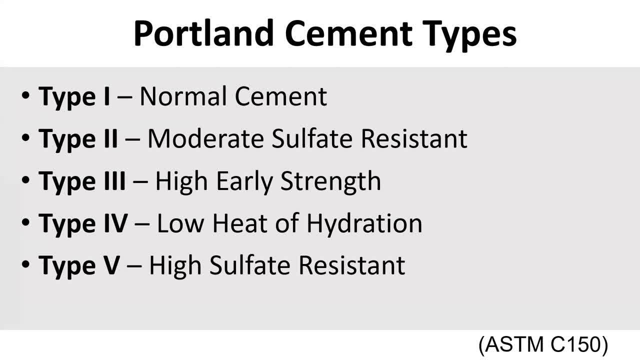 there's not a lot that make that are capable of making a type 5 cement. so what they'll do is we'll take a type 2 with with a class F fly ash usually, even sometimes even a class C, and we'll just do some testing to see how sulfate. 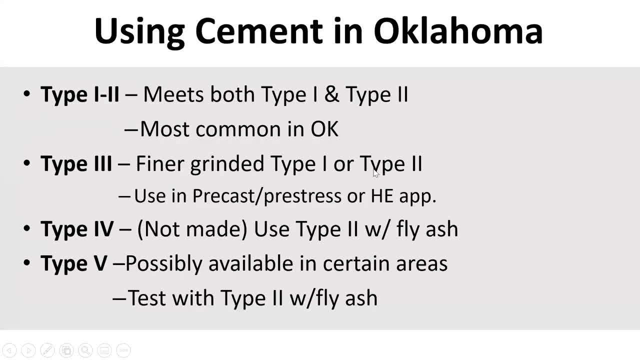 resistant. it is so in Oklahoma. I, I again, most of the cements are going to be a type 1-2, meaning it meets the requirements of both the type 1 and a type 2. that's the most common in Oklahoma. type 3: there's a couple plants that make a type 3 cement so high early. 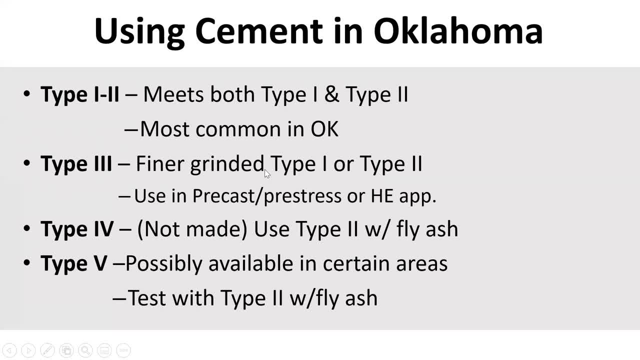 age age cement. this is typically going to be used in your precast facilities, pre-stress facilities. you may see it every once in a while on a- they don't do a lot of high-rise buildings, but you may see it on that- but not normally in. 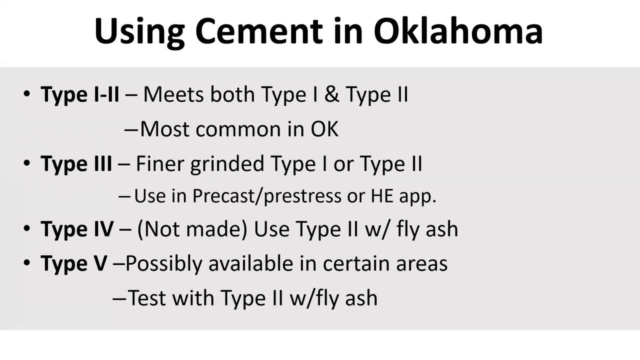 Oklahoma. you just see it on other places in the United States that have more, more type 3 cement, again type 4 it's just not made use, a type 2 with with fly ash and then a type 5. it is possible to maybe get it. I think Ashgrove cement up in Chanute has made a. 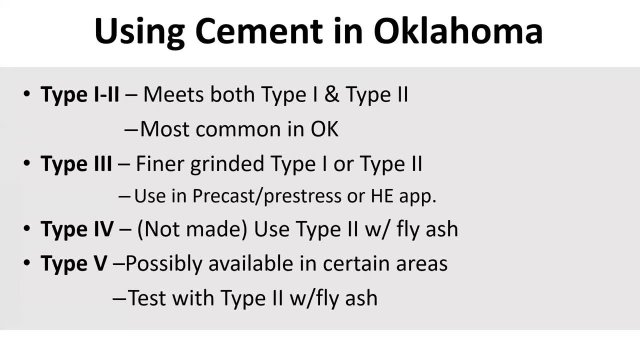 type 5 cement in the last five years. Bootsy cement over in Maryknoll, Texas, which is kind of by Sweetwater they are. they have made a type 5 but it's just not as they're. they read in their plant and so they actually I think they're. 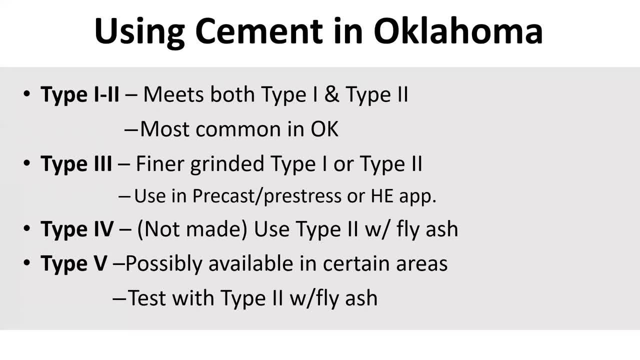 oil. well, cement technically meets a type 5, but it's, it's better to just really, from what I understand, is neither one of them- unless they've changed their, change, their, you know their fillings- they really don't want to have a type 5 cement in their silos. that earlier just sell you a type 2 and then just have you. 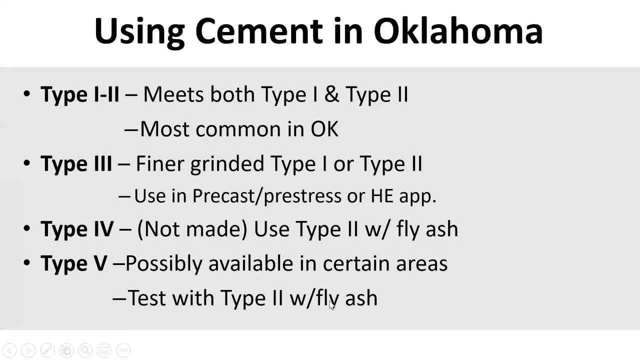 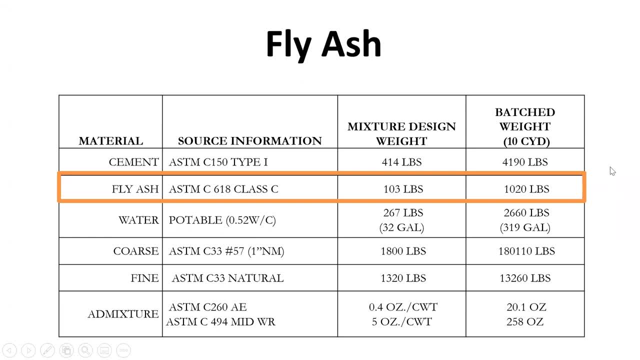 know, and then use fly ash and do some testing with it, because it really messes those spaces, but they could change, okay. so I'm not, you know, I'm not their advocate. I don't know, I don't represent either one of those companies. so you know, but that is what has been communicated just in the last couple. 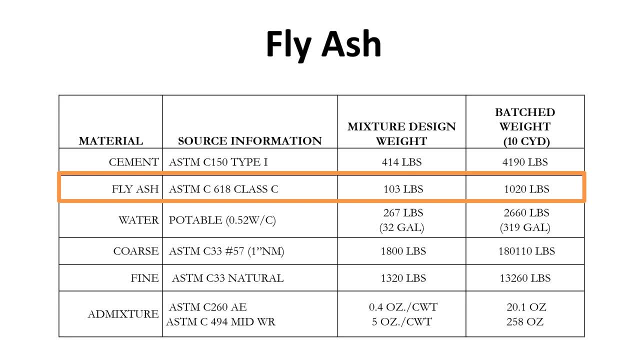 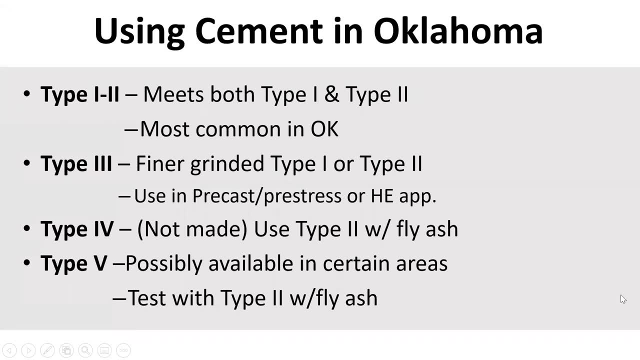 years for sure. but they may, you know, they may open up and make, make a type 5, but I doubt if they will. it's just not not, not used very much. there's only just there's really just a few cement plants around the whatever zone. so you know, it's just really doesn't matter much. there's just not as much as not very much. there's really just a few cement. 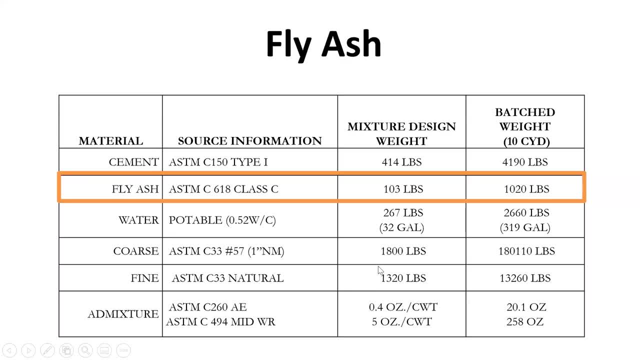 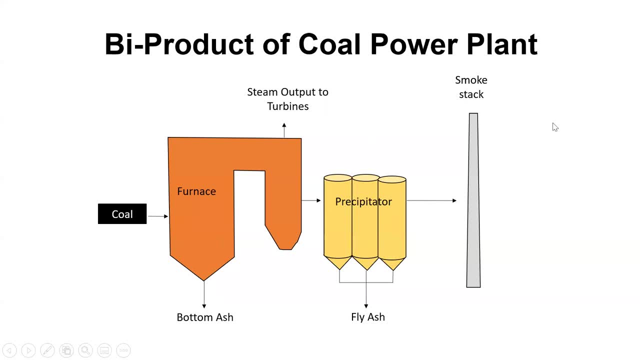 plants that make it. We talk about fly ash. Fly ash is actually a byproduct of the coal power industry. So whenever you go and you your electricity at your house, it's actually put through a furnace. that coal gets burnt up and you have two types and it generates. you know. 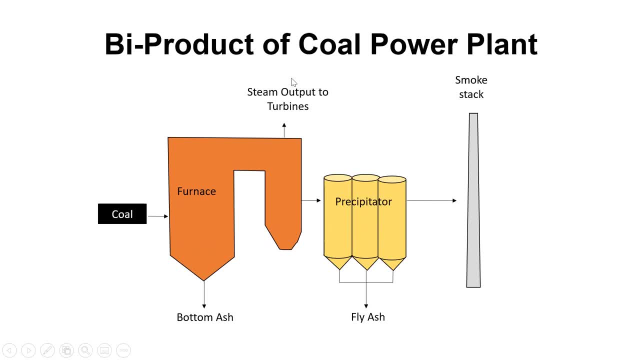 that has steam, that gets the output, that generates the turbines, Well, that's great, and everything but this coal that gets you know it's combusted, it's burnt up. you actually have, um, you have two different things that are happening. You have your bottom ash and then you have fly ash. So if you 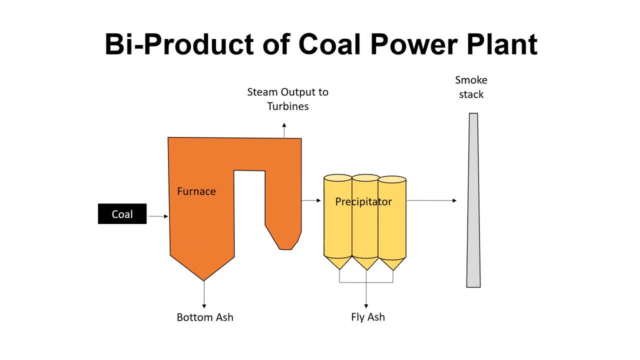 ever went out, maybe with a brush pile and you burnt some. you know burnt some, some limbs and stuff. it's very clear: whenever you watch that brush pile go up, there's some that you know a lot of people don't know about And they're going to say, well, why did you burn that brush? 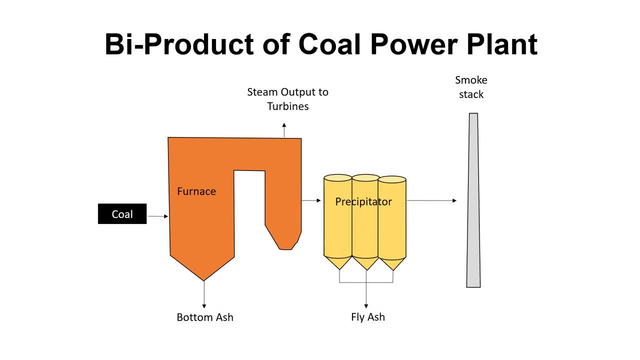 pile And you know. that's why it's so important that you burn that someanya coal is burning it, Because it'sib very stealing. it's been PMC. You haven't beenmouthed so in our day and age, when he wasn't lot of that. ash is on the is on the bottom, it's on the ground, and then there's also ash that flies. 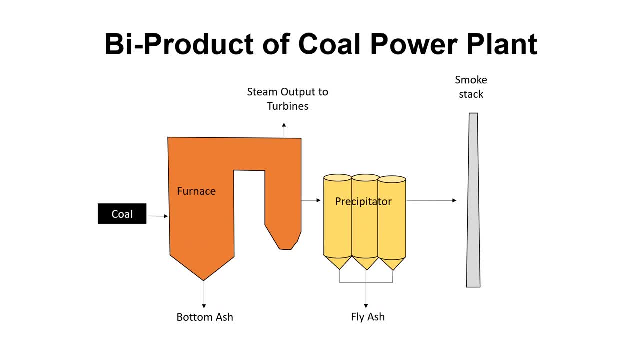 upward. that's literally what this is, the bottom ash, you know. just it's heavier, it flies down and then the fly ash goes upward and it gets caught into precipitators. they have funnels and everything, so it just doesn't just go out the smokestack, they collect it all and they say: oh my gosh, what. 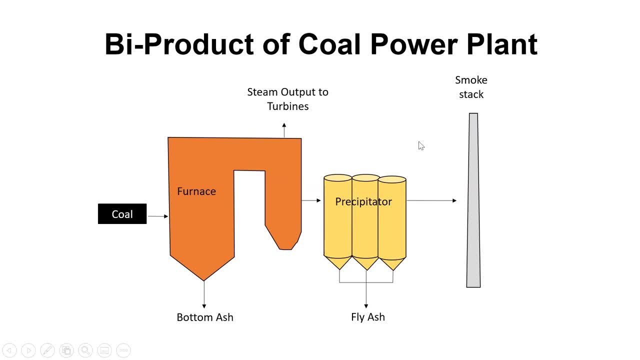 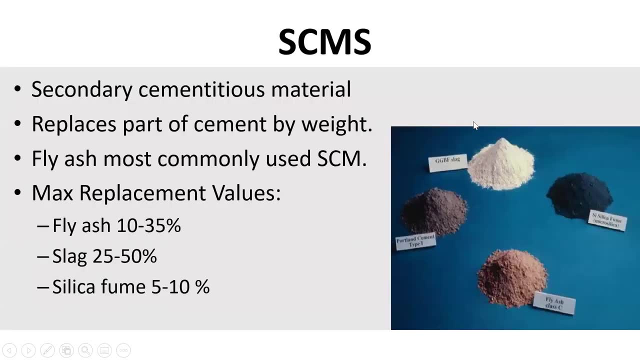 are we going to do with all this? you know, ash, that that flew up in the air. well, we're going to call it fly, ash, and we're going to and let's see how good it works in concrete. and they found out it worked really well. you could actually take out a little bit of portland cement and you could add. 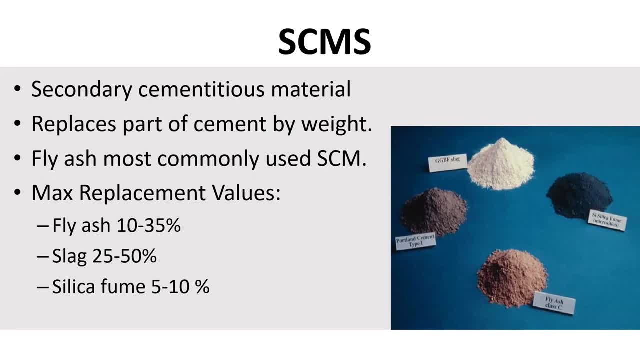 um, you know fly ash, and the same thing happened actually with slag, so slags from the steel industry. and what they said was: aha, you know, i can take this, the slag, you know this, this, this byproduct from the steel industry, i can take it. i. 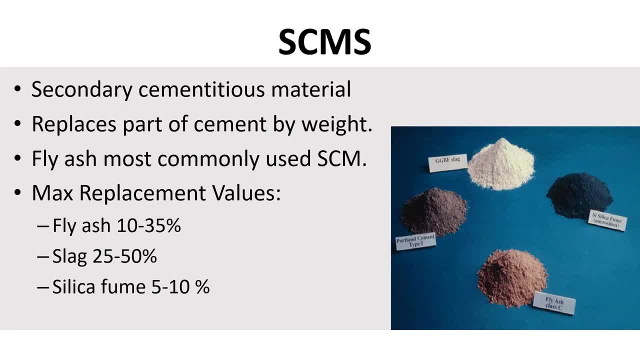 can regrind it and then i can put it in concrete and it works really well and it's a you know, and both fly ash and slag are normally a lot more economically cheaper than cement. cement's usually one of the highest ingredients because you're fully manufacturing it. um, silica fume is actually. 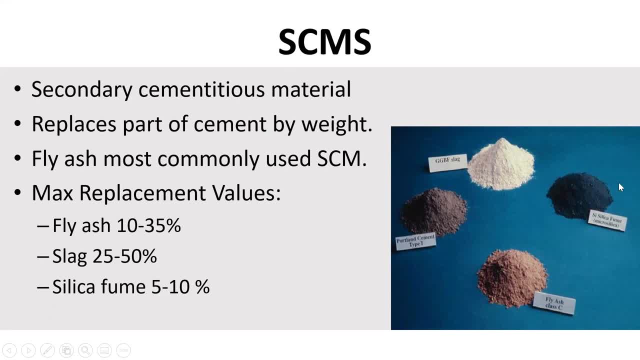 from the silicone computer industry and it's a byproduct too and so very similar to what you think of with fly ash, and so they'll just collect it all and this silica is very micro fine, really, really, really small particles, and they'll take all this um these different scms, and they've used them in concrete, so normally you 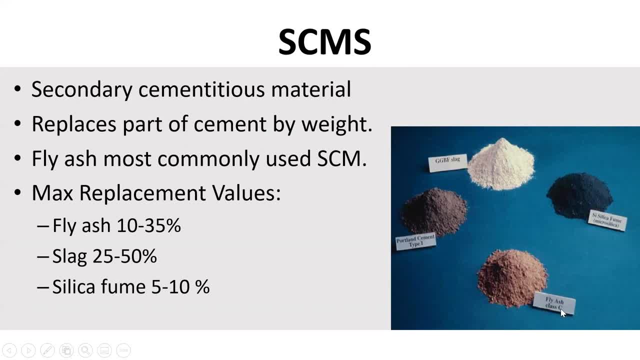 just have one scm. you usually have a fly ash. either it's a fly ash or it's a slag, or it's a it's a, two different classes, either class c or class f, based on the calcium content of them, and one act and then so, in that the differences mainly are how they react. 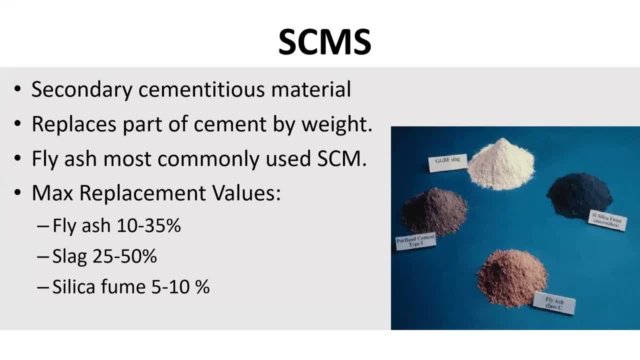 um how they perform in concrete, and so for fly ash, usually between 10 and 30 percent, 10 and 35 replacement is really common um so you're literally you know, say it's 10 replacement, so you're going to take. so in general, you know if 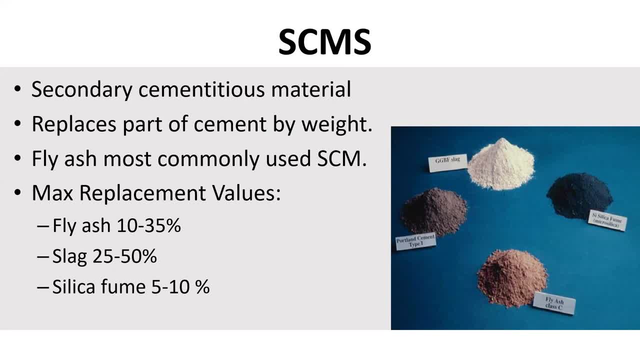 it's. if it's 100 portland cement mix and you want to replace 10 with fly ash, you're going to take out 10 of the cement and you're going to add 10 of fly ash. that's kind of what the replacement value. 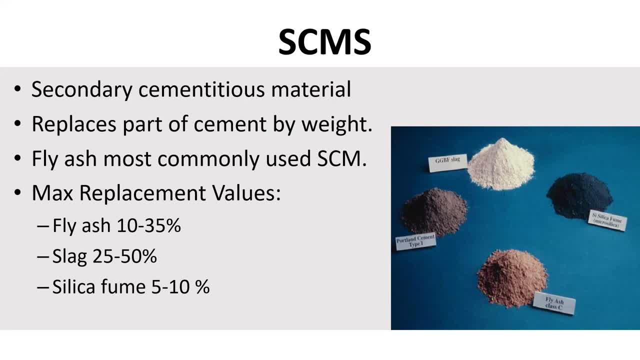 is about. so your mix is really. you know, the result is you have 90 portland cement and 10 fly ash, so together it's still 100 percent cementitious materials. but um, that's kind of the difference and that does save you some money for your concrete and it does produce it. um, you know, it can't improve the properties. 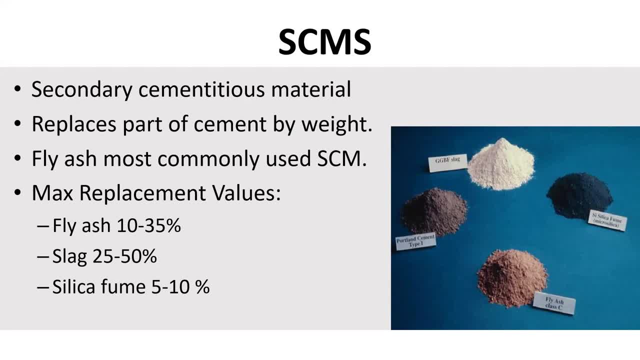 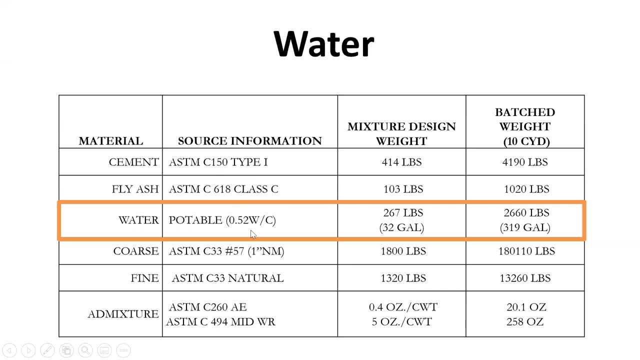 the performance properties of your concrete, whether it's durability or workability. it can't improve it. water is something that's sometimes overlooked. you really don't want to use super dirty water. you want to use something that you can drink. you want to use something that you can drink. 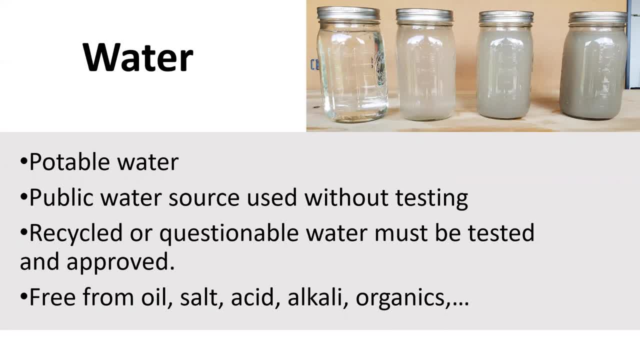 so most public water sources are going to be used without, without needing to be tested, recycled or desirable water. you know it really needs to be attested and approved. so this is a couple different things we do because it will be without adding pesticides. you know we do this with 30 or 30 Pereg RBIS, the 20 or 30% formula for you. 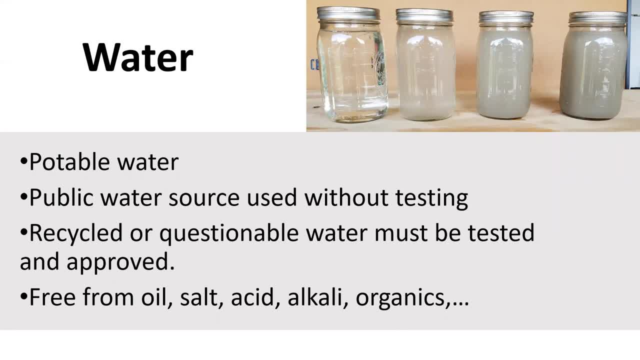 approved, so you know you need to go out. if there's anything you don't wanna, you wouldn't drink the 20 or 30% formula for you, and or if it's recyclable water, you really need to go. don't want to drink. how long it was. 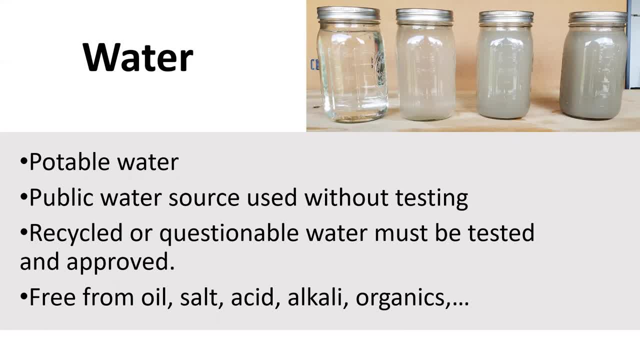 out and test it, make sure everything's gonna look good. الب인가 flora: you really need to go out and test it. make sure everything's looked. green raps is need to go out and check. but they're it. it's for involved persons don't want oil, salts, acids, alkalize prunes, organic. You don't want to do it forever just to see if everything. 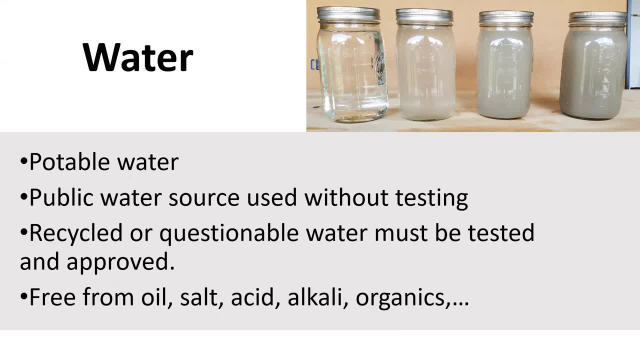 salts, acids, alkalis, organics, anything that's going to change the strength of your concrete, change the area of your concrete, the workability. You really want something that is going to be pretty low maintenance. So you kind of have to be careful when you talk about recycled. 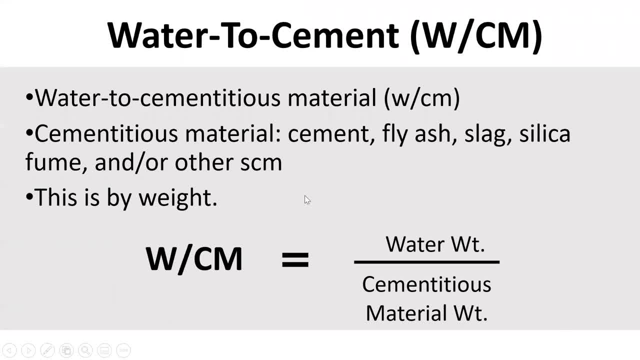 water, You have to have kind of a system in place. Well, usually when you talk about water, people focus a lot on the water to cement ratio. So how much water do you have compared to the amount of cement that you have in that concrete? So it's kind of like, if you think, 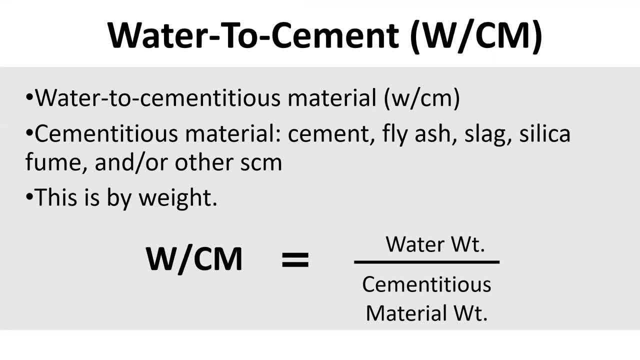 about painting and you do whitewashing, you whitewash. So if you keep adding water to your paint, can you can get more and more paint out of it, But eventually you get to a certain point where You know it's really water that you're painting on that, say, that fence that you're painting. 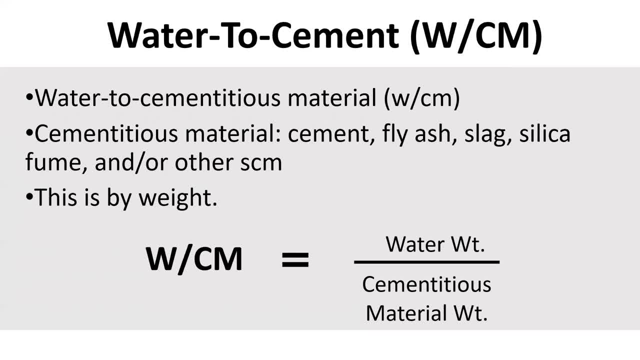 on that wall or whatever you're doing, And so you don't want, obviously want water, And so it just depends on how. what degree of whitewashing do you kind of want whenever you're painting? So that's kind of what you're doing with cement: The more water you add. 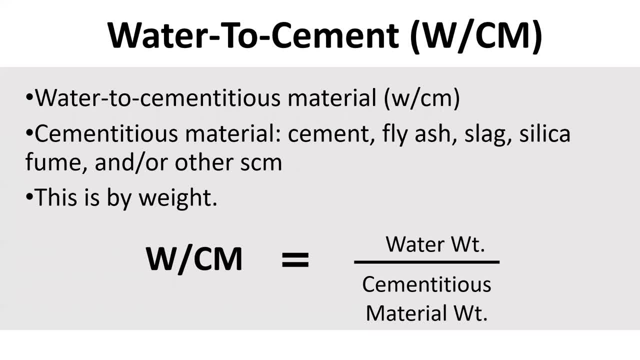 the more you're diluting your cement So it has less and less impact. So you're going to have lower strengths normally and you know it's going to change your setting time And you could even have cracking issues because the concrete's not going to have. 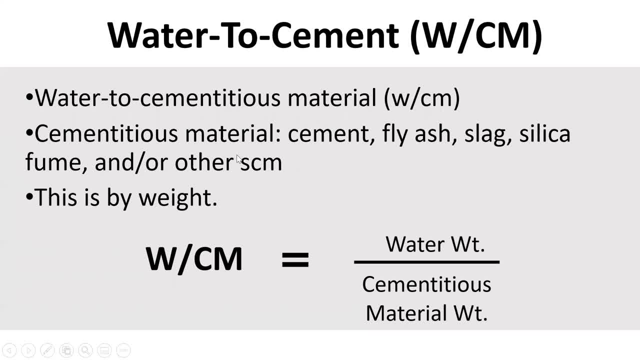 those, those good internal stresses, So all times now. so they've called it a water-cement ratio, they call it the water to cementitious material ratio, either one, they're kind of interchangeable. But just realize that cementitious materials, you know there's, there's a lot of different types of cement And so there's. 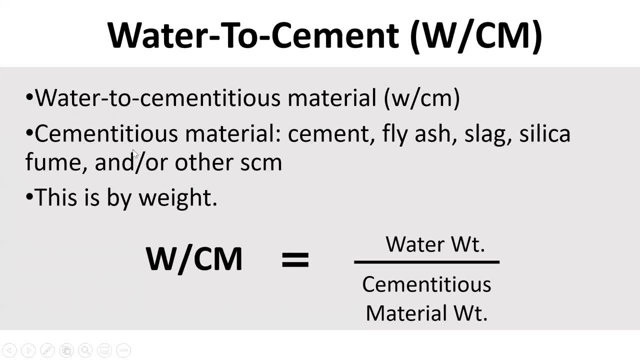 It's going to be the cement, the fly ash, the slag, the silica fume, et cetera. And this ratio is done by weight, So the weight of water divided by the weight of your cement and slag fly ash. 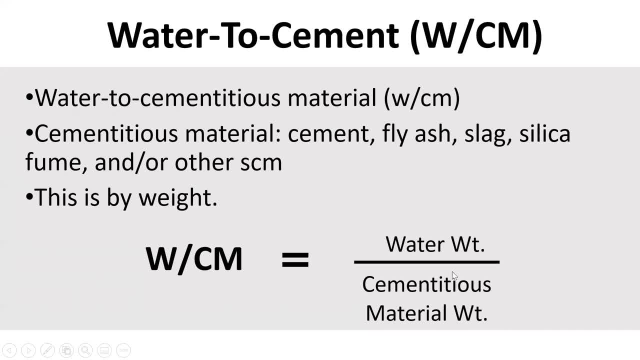 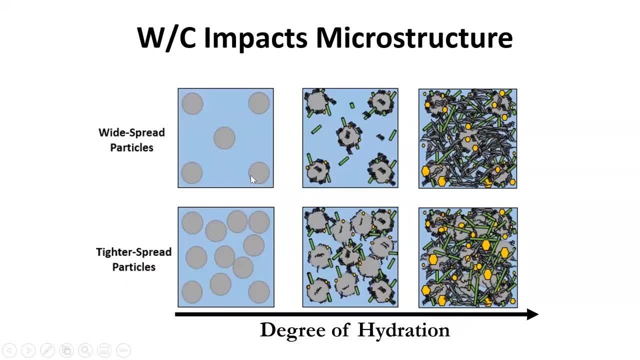 everything that's used in that specific mix. that is your water-cement ratio, So it's by weight. So how that kind of looks. we talked about whitewashing and painting and stuff. You know, if you have less cement and more water, your particles are going to be farther apart. 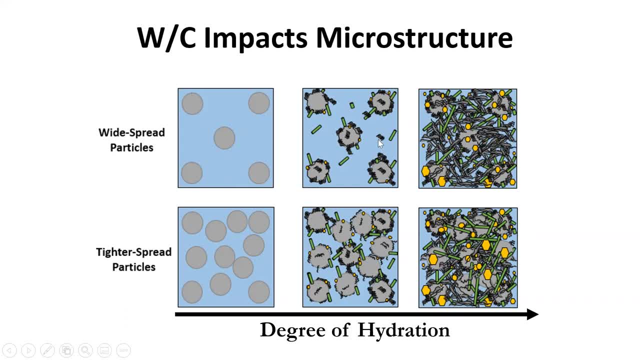 Your cement particles are in the water solution And so over time, because it's a chemical reaction between cement and water, they're going to produce product on the outside and they're going to have a harder time to connect. It's going to take longer these bonds to connect all these particles together with these products. 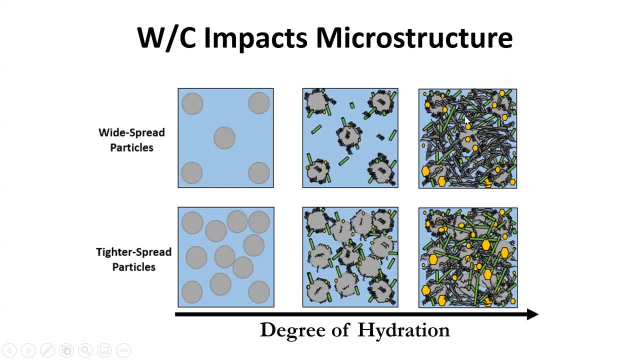 It's going to take longer. It's going to take longer. It's going to take a lot longer to get to initial set and final set And then over time, your strengths are just going to be weaker because it takes a lot more to extend, to get that bond from the cement particles. 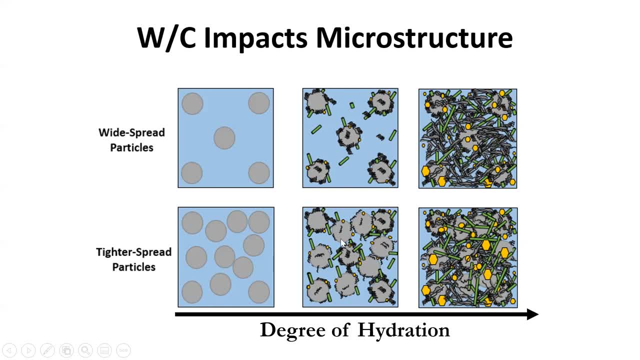 And if you have a tighter bond, like you see here, it's going to be easier to bridge, to get to these cement particles and you'll have a much tighter matrix, a much tighter pore structure of your concrete. So we'll talk about aggregate. 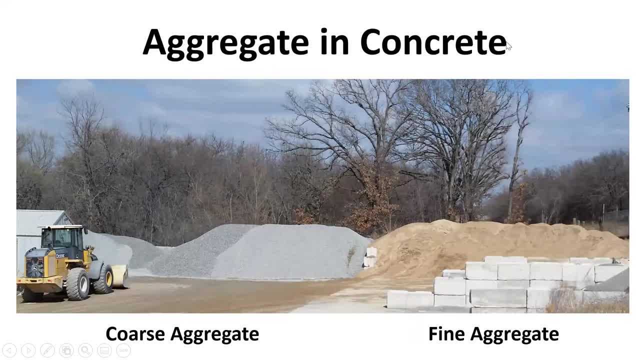 Again, coarse aggregate, fine aggregate. they make up over 60% of the concrete. I've seen some where it's actually up to 90%. You really want you know. you have your coarse aggregate here, you have your fine aggregate here. 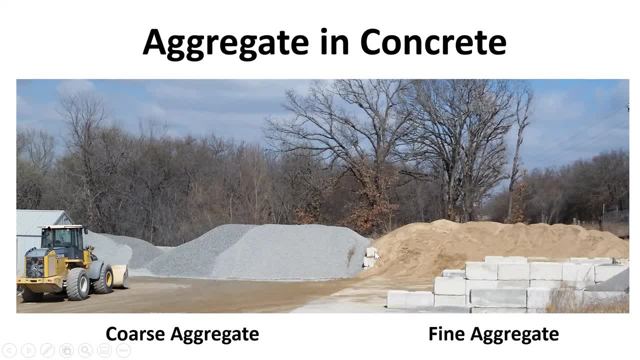 You really want this wall to be built up higher so that you don't get contamination, because you want- you know, you want- coarse rock whenever you take a scoop with a front-end loader. You don't want, you know, coarse aggregate with a little fine aggregate. 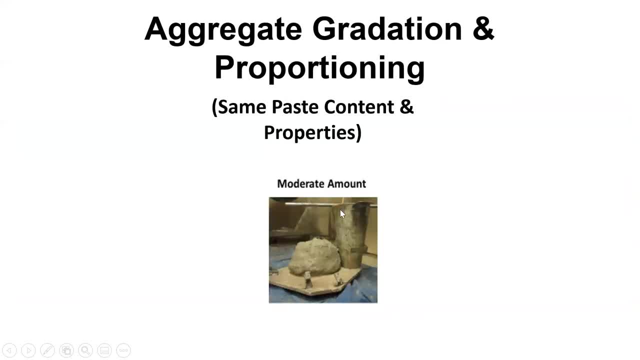 So you know, just kind of be aware of that. And aggregate is a huge deal. Not only does it make up, you know, 60 to, like I said, 80,, 90% of the volume of the concrete. 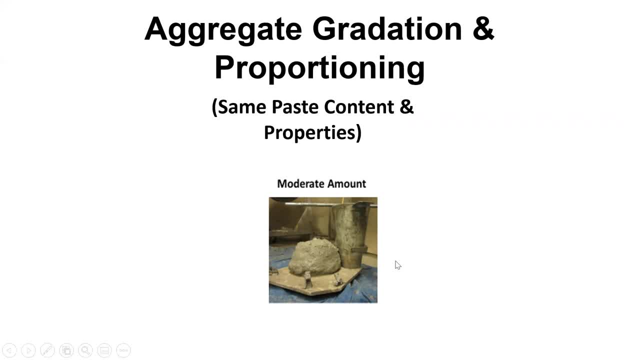 but, like you see, here, with the aggregate gradation, I'm going to show you five mixes And the only thing I'm doing differently is I'm changing up the rock and the sand, changing the gradation, So it's the same amount of cement, same amount of water. 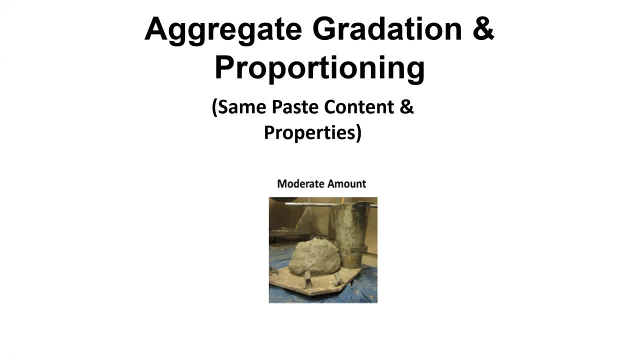 Same amount of admixture. The only thing I'm changing is the aggregates, how they're proportioned, And so this exercise kind of explained to you how important aggregates are, and the gradation. So this is a basic, moderate amount of both rock and sand. 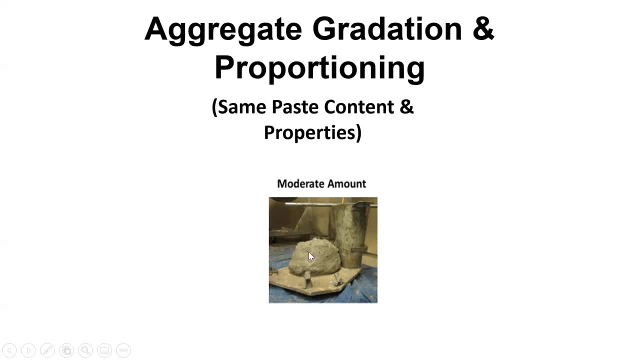 And so this is for a five-inch slump. You can pump with it for a bridge deck, You can use it for a floor slab. It's a very typical mix And I use a slump test here because that's the most commonly used test to kind of communicate the workability of concrete. 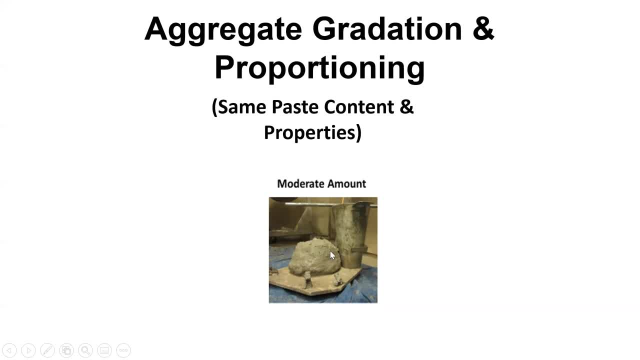 So this is a five-inch slump here. It's a very good mix, You know, if you have you know. so what I did was I took out a little bit of, took out some rock, put in some sand, put in a lot of sand. 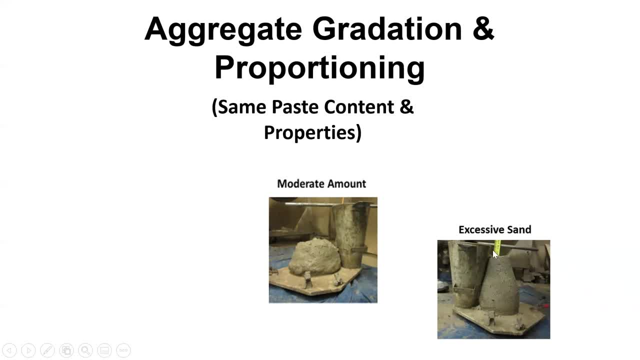 And if you have too much sand, what a lot means. if you have too much, then you're going to get a nice stiff mix That's actually not only stiff but it's sticky and it'll stick to everything. This is so what for me, in a five-inch slump to I think it's down here- at like a two-inch slump. 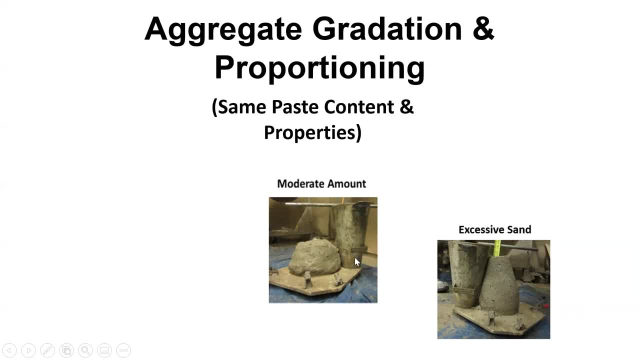 So again, only thing I did these: they're completely different work abilities. This is great for floor slabs, This is not. you may not even want to pave with this, even though it is a two-inch slump. You may not even want to pay because it's so sticky. 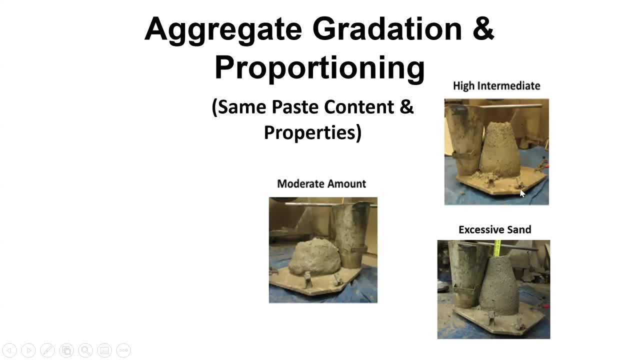 You can also have a high intermediates. We have a bunch of three-inch slumps. We have a three-eighths inch chip put in in in there. So you take out a little bit of rock, you put a little, you put a little three-eighths inch chip like a little intermediate. 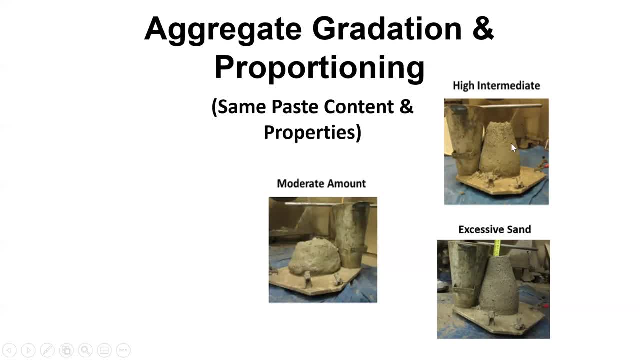 And all of a sudden it gets stiff too. So it's not sticky like the sand, but it's really stiff, And so this is actually more of like a two and a half three-inch slump If you don't have enough sand. 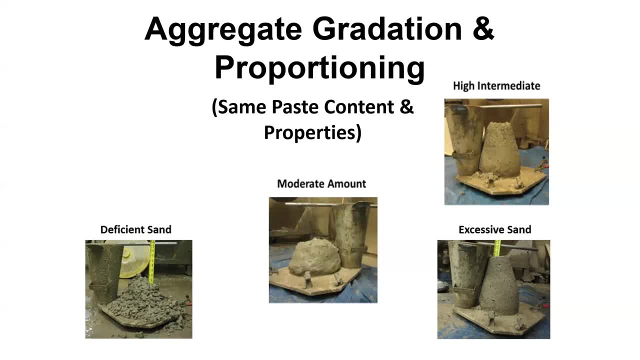 So if I take out all, if I take out a lot of the sand and I put in a lot more coarse rock, you're going to get something that looks like a bunch of rocks covered in paste. So this is a seven and a half inch slump. but you know, the cohesion looks absolutely horrible. 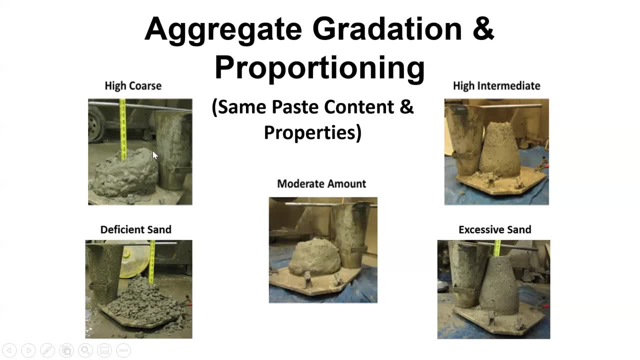 And then if you take out and you add more coarse rock and you take out some of the and you don't have enough, you just keep adding more and more rock to it, You're going to get to a point And you may have a, you know some, some enough sand, but you don't. you have too much, way too much rock. 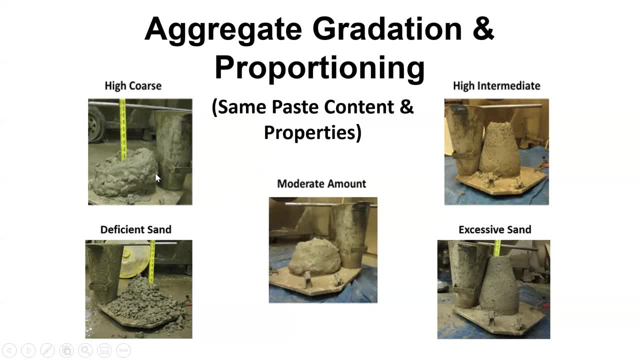 What's going to happen is you're going to get a lot of segregation. You know those are these rock particles and just kind of want to separate. There's just too many of them. So you kind of need like a almost, like a well graded distribution of aggregates, almost, And what that well graded kind of defines. 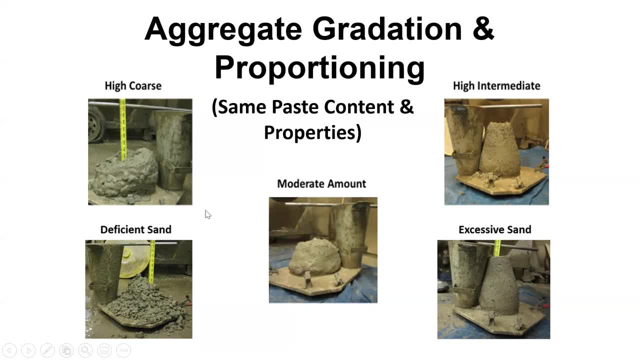 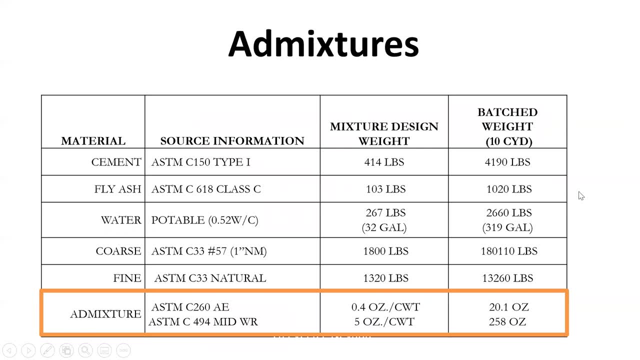 You know, I think of the tarantula curve that I developed And that kind of helps to kind of communicate where some of that's at, And we'll talk more about the tarantula and stuff in a later class. So last thing is add mixture. So it's very common to use air entrainment for freestyle durability. You may also use a mid range water reducer to improve your strengths and your work ability- mainly your work ability- and it will increase your strengths normally too. 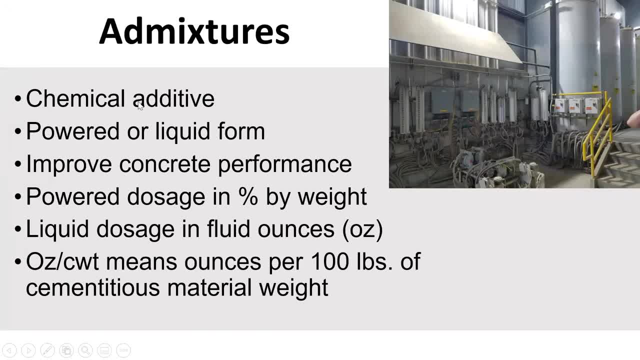 So chemical additives are usually either chemical additives Is what I'm referring to, So you have powdered or liquid form, And they're. these additives are usually added to improve the work ability of the concrete. That's what they're incorporated for. Powdered dosages are usually percent by weight. liquid dosages are in fluid ounces, So ounces per CWT, that is that actually means. 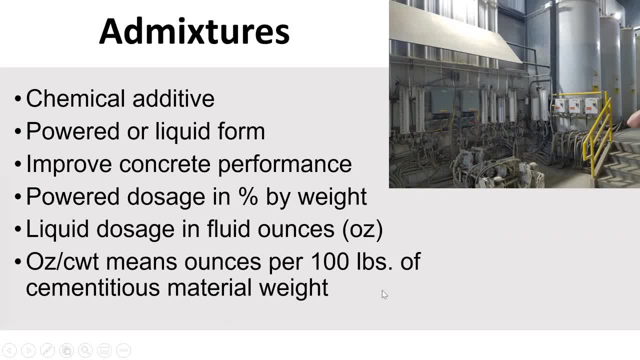 100 pounds or ounces per hundred pounds of simple water, And that's what we're referring to as cementitious material. so that kind of helps. So if it's, you know, four ounces per hundred weight is what it's referred to. That means there's four ounces per per every hundred pounds of cement in that mix. So if you have, 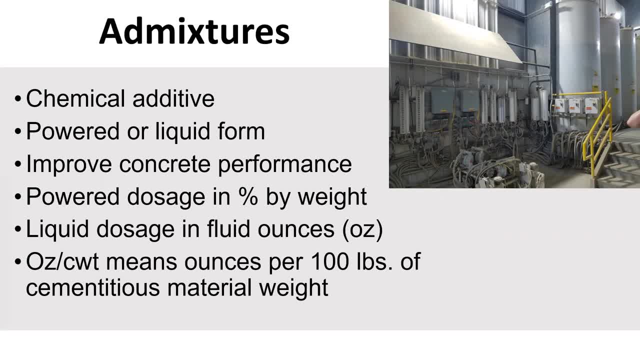 You know, 400 pounds of cement or cementitious material. that, and you know, you're proportioning based off of four ounces per hundred weight. Then that means that you're going to have at least 16 ounces per yard and your mix So four times for. 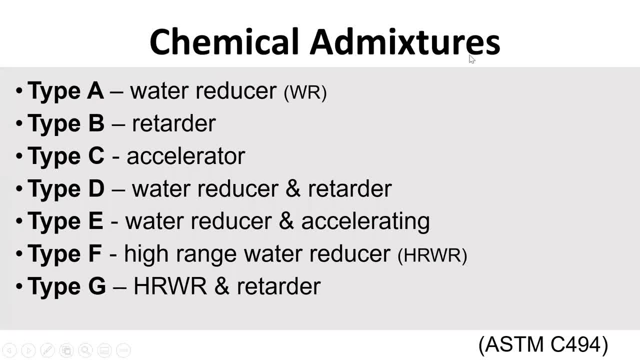 In for a STM: see for 94 chemical add mixtures. There are a variety of different types. There's even a type s that I don't know why I left off, but it's down here also. So type a, Type D, type E, F and G are all water reducers. 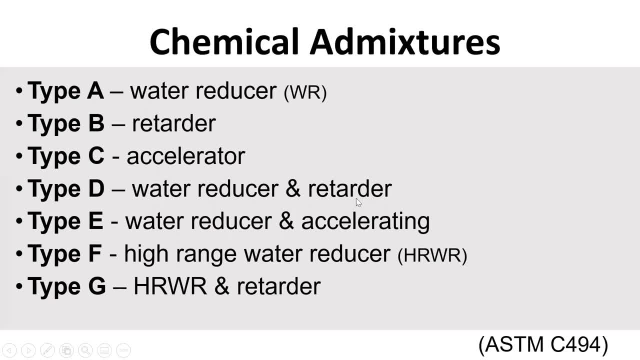 Some also Are accelerators, a retarder, and then other ones like a type F and a type G. Those actually Drastically improve the workability of the concrete even farther than just a type a, D or E. So they are, you know, type F or type G. 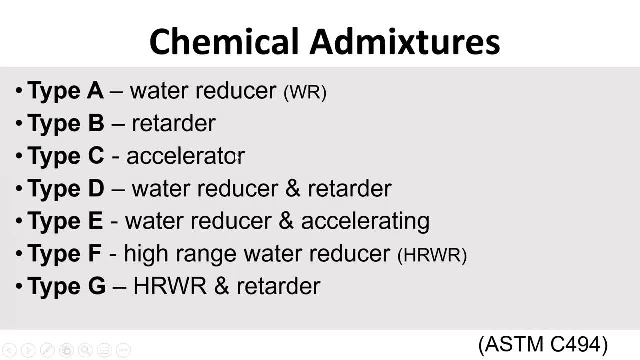 You also have a type B or type C. That's just our accelerator or just a retarder. So they may be a combination of a water reducer and a retarder or an accelerator, or they may just be one. you know, they may just be a water reducer or an accelerator. 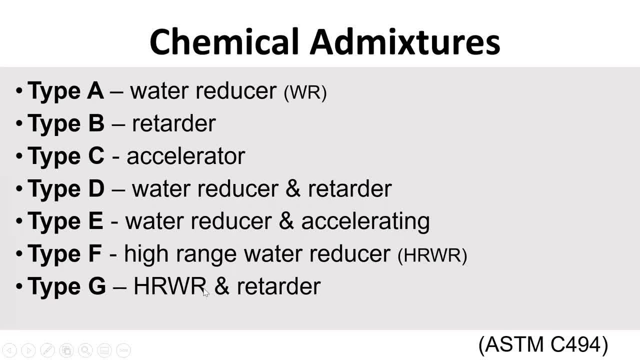 So if you think about like a super plasticizer, that is very similar to a high range, that is same thing as a high range water reducer. So you know, or a plasticizer, super plasticizer, super P, those are all the same terminology And they are technically all water reducers. 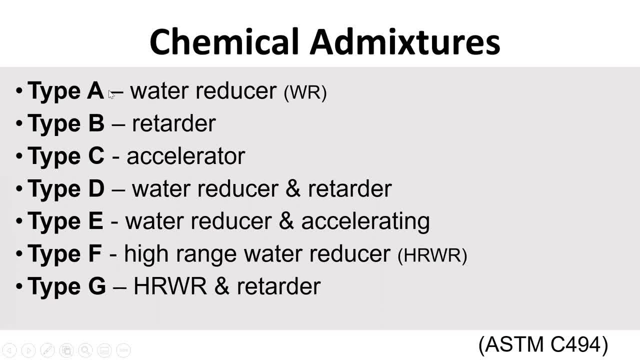 But this is more focused. the type A, D and E are more of like what you think of as like a normal or a mid range where they, where they have, you know, more of a slight to a moderate workability improvement, as opposed to like a type F or G which have a major change. 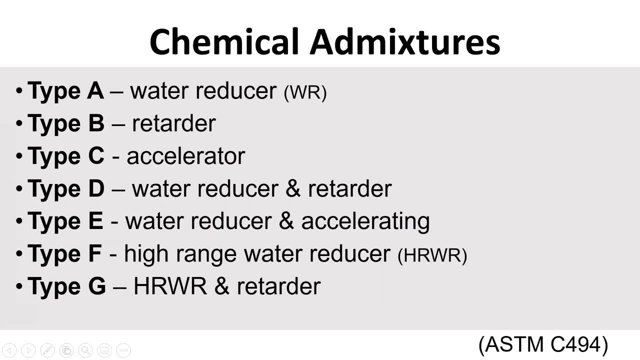 they go from being, you know, such as like, for example, a really stiff two inch slump mix. to you add, say, four inches or four ounces of a high range water reducer, or you know, and all of a sudden you're at an eight inch slump, And so it's extremely flowable difference, And so that's.